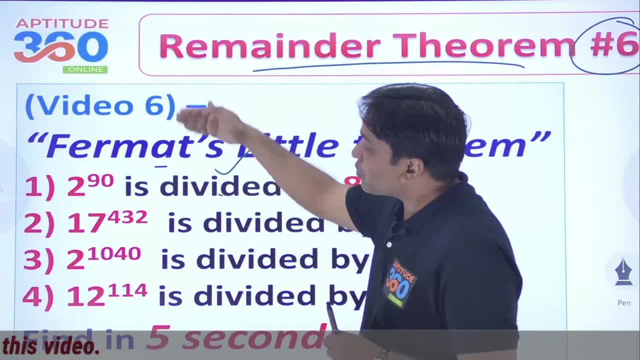 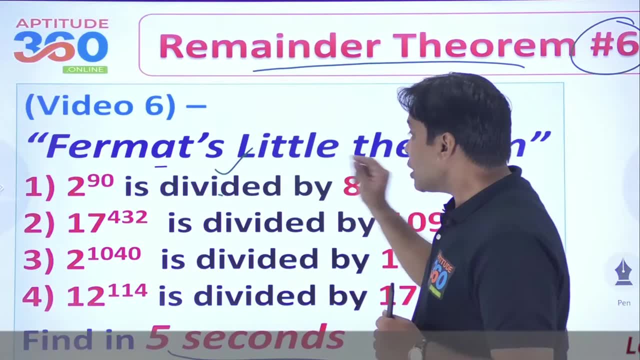 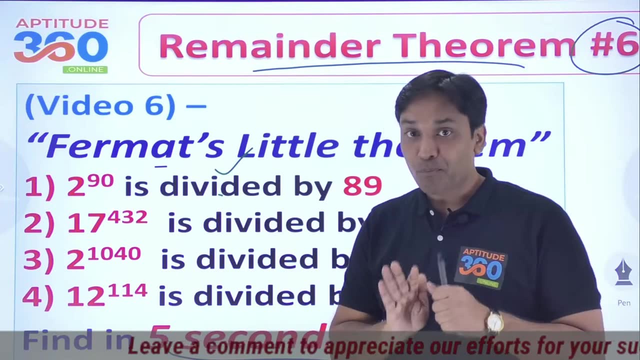 permits written theorem and how can we utilize permits theorem to to solve this, this, this kind of problem, right, and and i am kind of confident that once you have learned this theory, it may right. uh, having said that, i let us introduce what exactly is the theory out here? 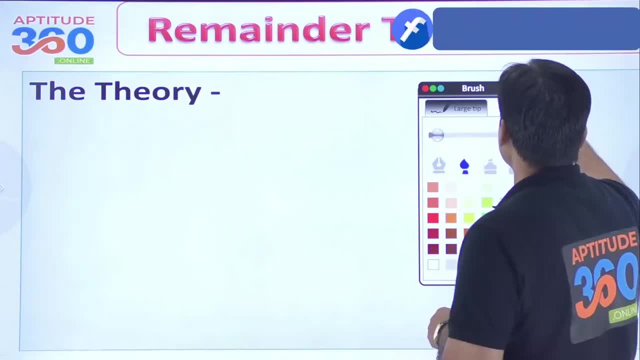 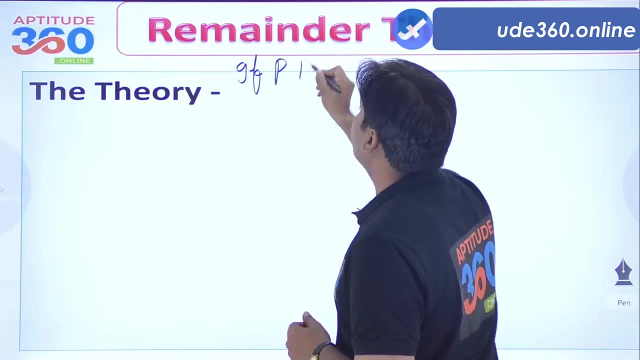 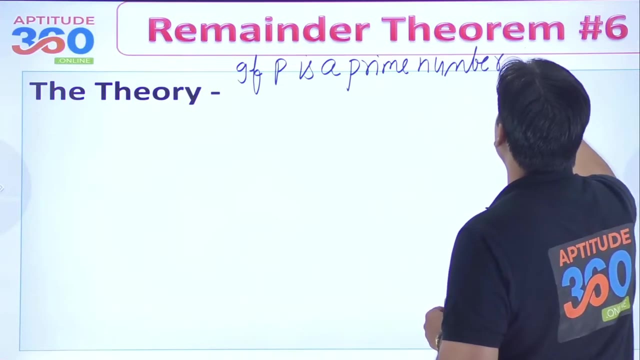 uh, this theorem is taught in in graduation classes of mathematics and i'm i'm gonna write that statement, uh, so that if, if p is a, if, if p is a prime number, if p is a prime number, then i would say that any number, any number, a. 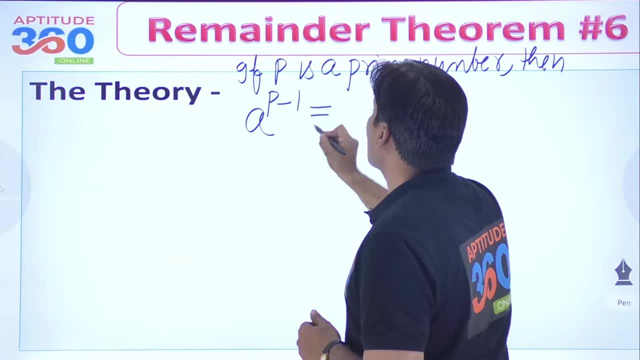 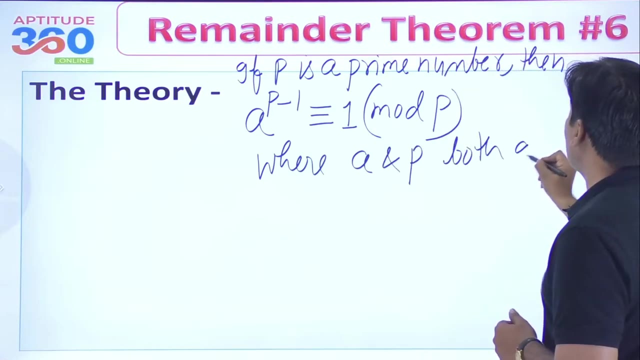 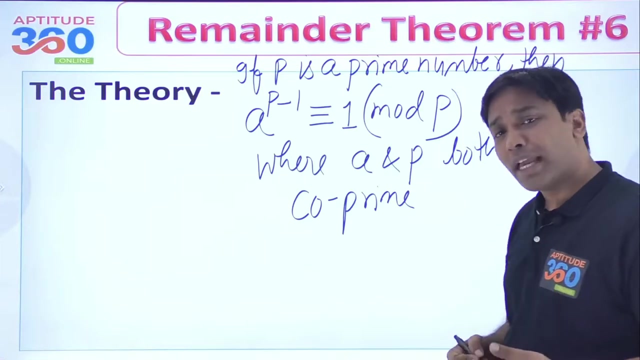 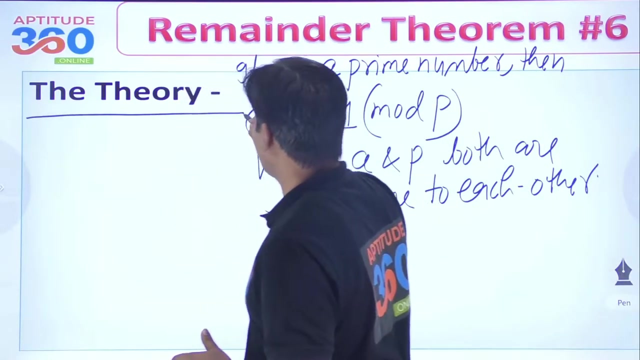 is to power p negative 1. this is congruent to 1 modulo 1 modulo p right where, where i would say that a and p both are, both are co-prime to each other. they both are co-prime to each other. what, what are we gonna do? we will be simplifying this entire thing over here so that, so that you. 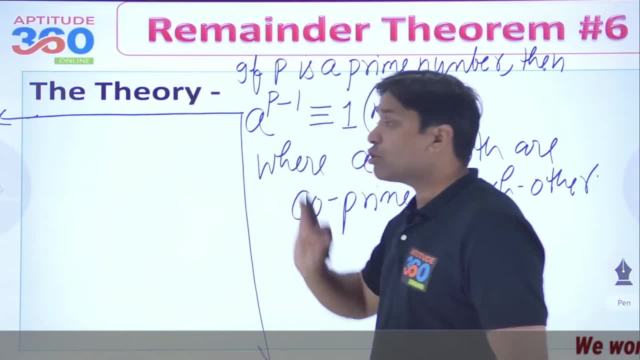 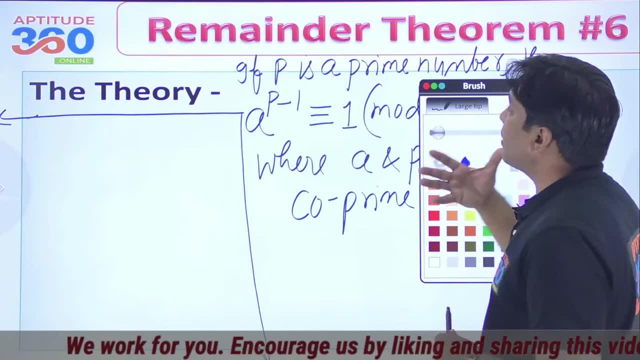 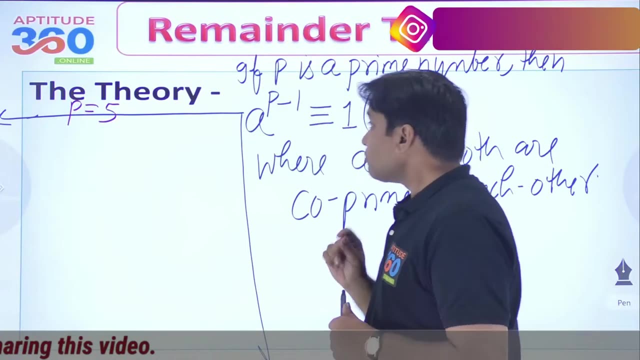 understand what is that i am talking about. here is a prime number, so we will take a prime number, we will. we will consider some prime numbers, let us. let us take r p over here. r p is 5.. p is a prime number, right. another very important thing is uh, this number. 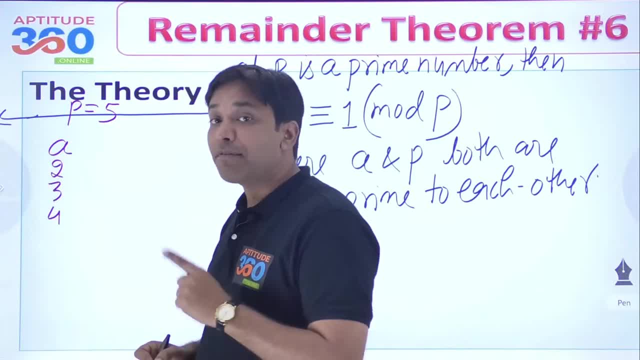 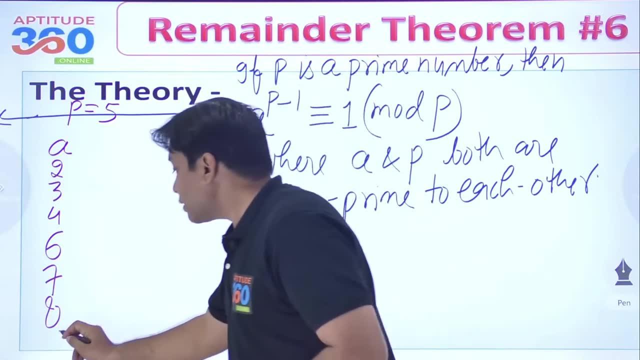 three and four, but we cannot take it as five, because five is not co prime to five, and then six, and then seven, and then eight, and so forth and so on. if you do not, you can take it nine as well, if you do not understand what is a co-prime. 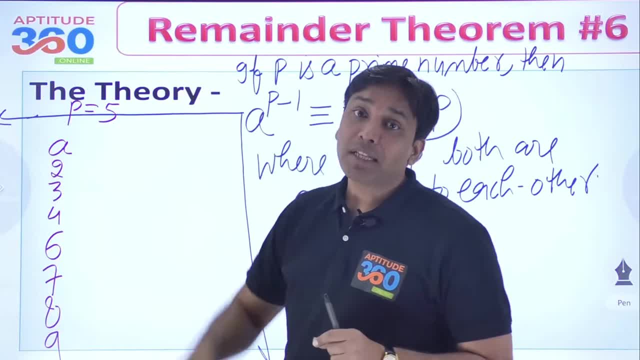 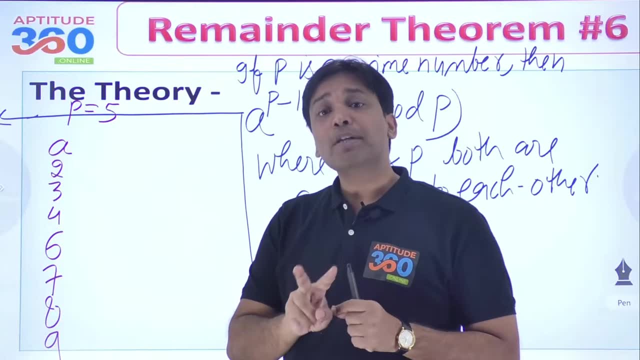 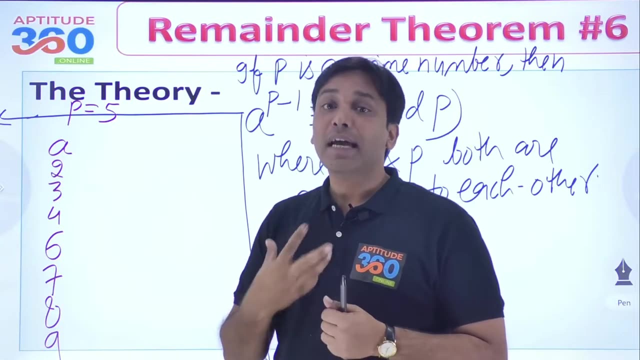 number. then go to this video and I have given the link in the description box as well, but make sure that you have. you have learned that particular concept. its very simple: two numbers are co-prime only when their highest common factor one, or we can say that these two numbers should not be having any factor. 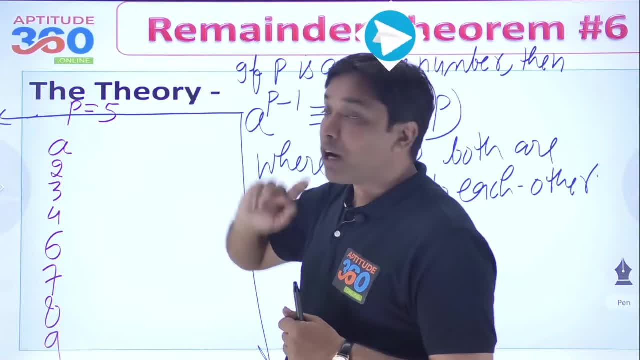 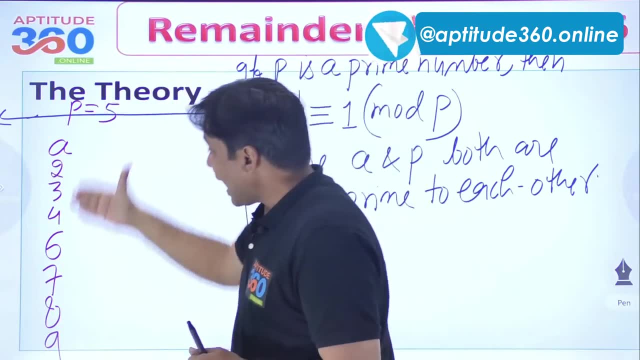 in common. okay, so if you haven't watched the video, then go and watch it. and I am continuing this discussion. I am saying that what if I have taken my prime number as five and- and I am taking a as these numbers? what is going to be then? 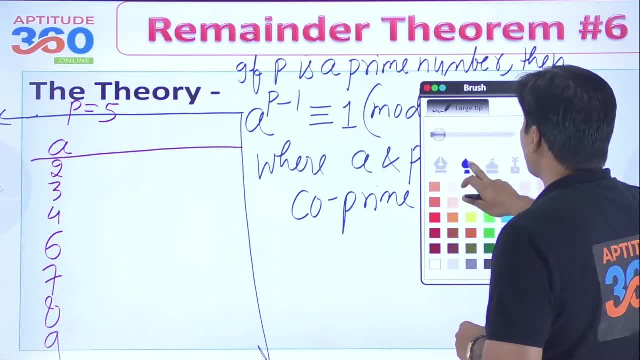 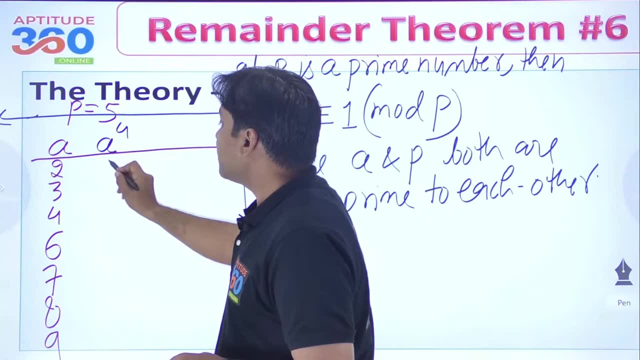 what is going to be A to the power. what does this problem say? we will have to take A to the power, p minus 1. so my, my a to power 4 over here, over here, will be 2 to power 4. 2 to power 4 is is 16 and 3 is to power. 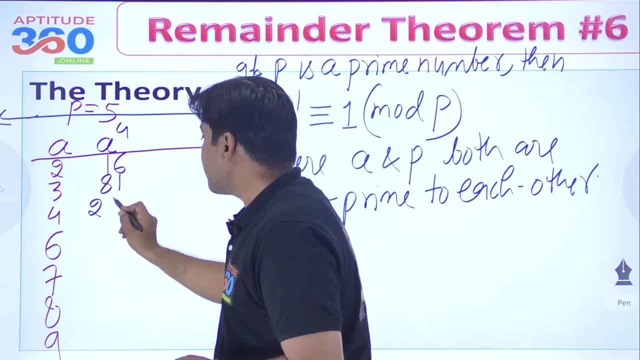 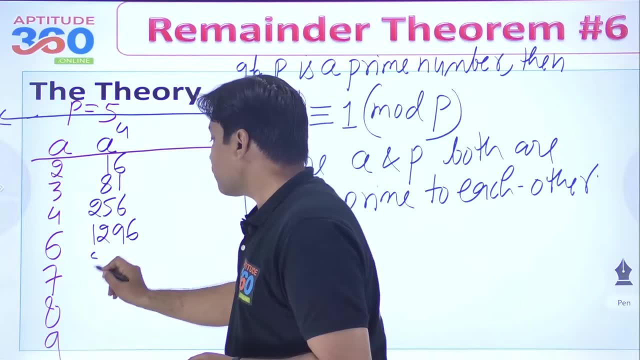 4 is 81, 4 is to power. 4 will be 256 right and 6 is to power. 6 will be will be 1296 and 7 is to power. 4 will be 2401 and 8 is to power. 4 will be 4096 and 9 square will be 656561. 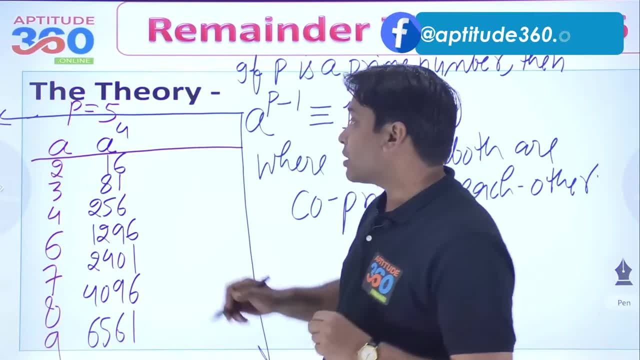 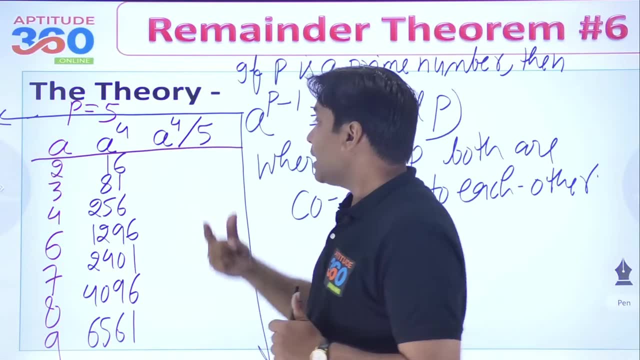 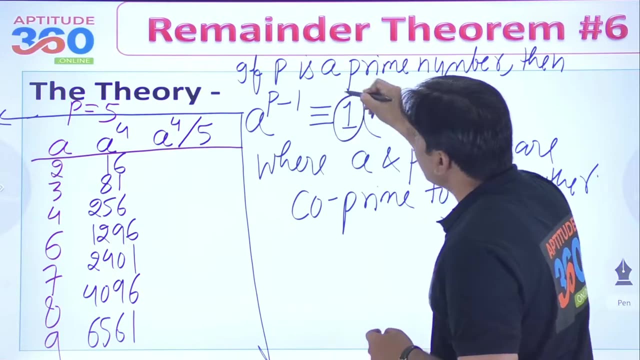 so these are the values now. look at one thing carefully now: if you divide, as to power, 4 by this 5- that is what he wants that- what will we do? if we divide this number by 5, then how much will be the remainder? this remainder, is saying here, will be 1. if we divide 16 by 5, then the remainder will be 1. 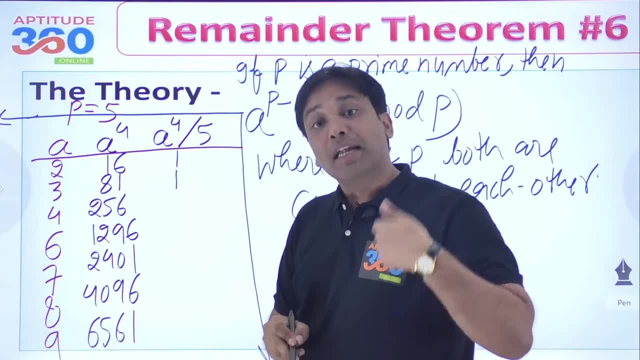 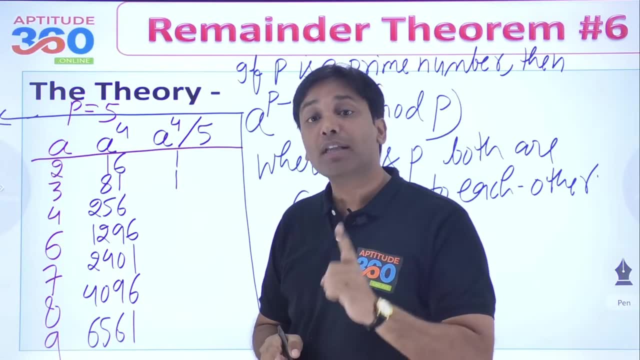 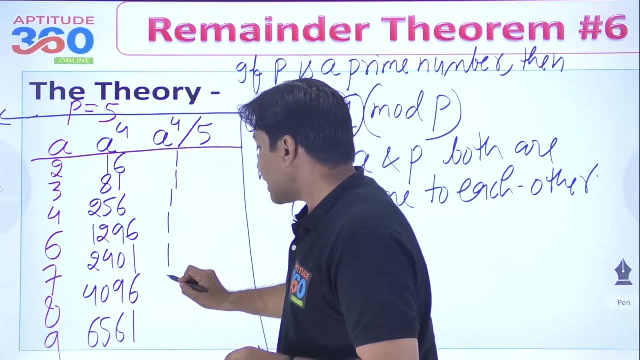 if we divide 81 by 5, then the remainder will be 1. you can see all these numbers. divide these numbers by 5 and see that the remainder will always be 1. this thing is not understood. that's, that's ok. but this thing should be understood here: that in all of these cases, 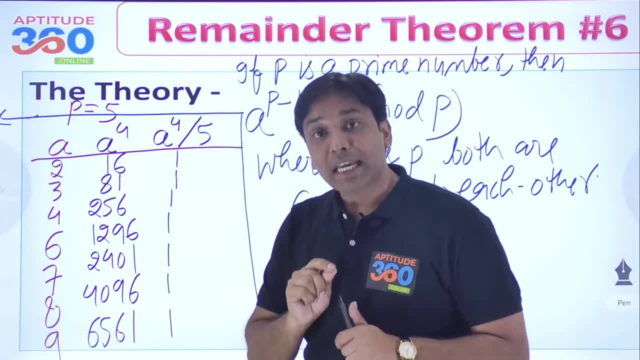 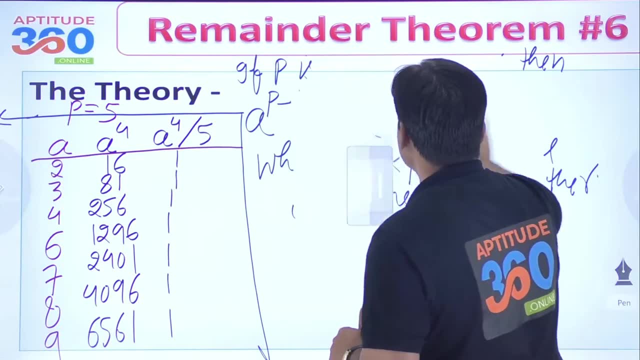 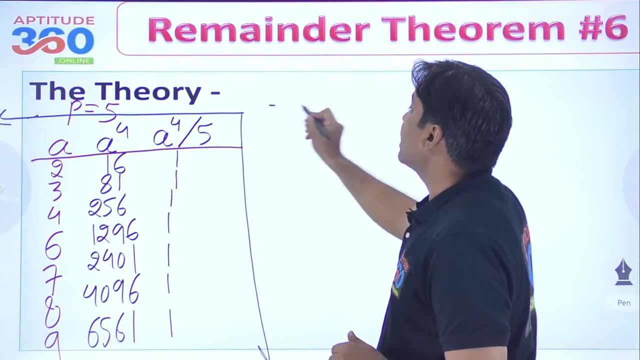 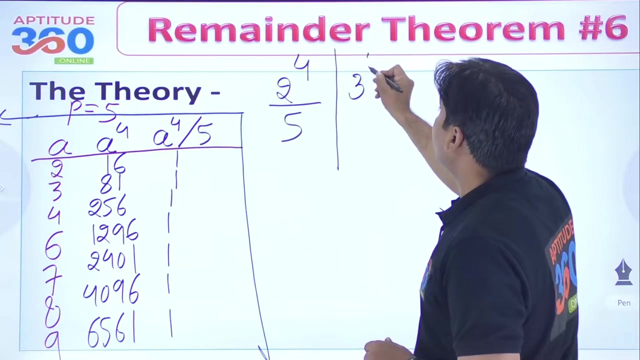 when we divide this number by 5, then the remainder certainly will have to be 1. it has a simple meaning. I explain to you here what will it do. it will simplify things. so if I say, if I say, two is to power 4 divided by 5, or all we have got 3 is to power 4 divided by 5, or four to power 4, 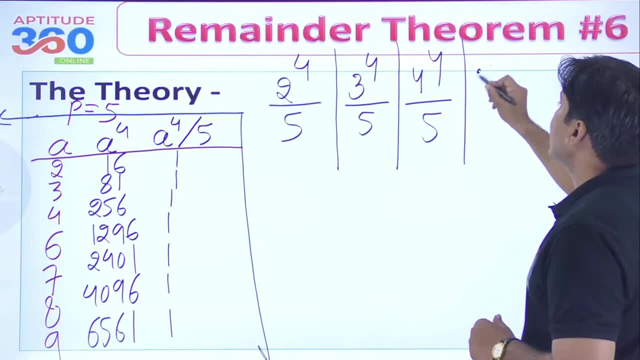 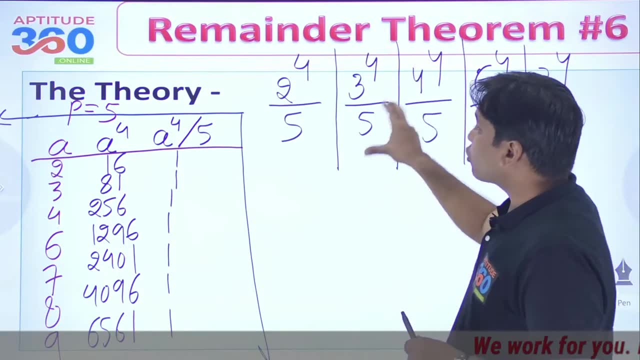 divided by 5 or 5. we cannot take. it can be: six is to power 4 divided by 5, sevens to power 4 divided by 5. if you divide three is to power four, five, five. so then you will come down to one, if you 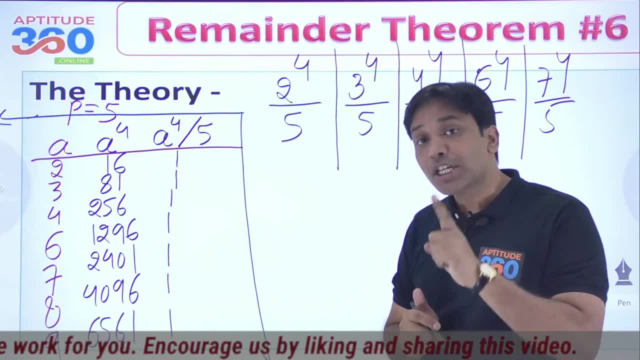 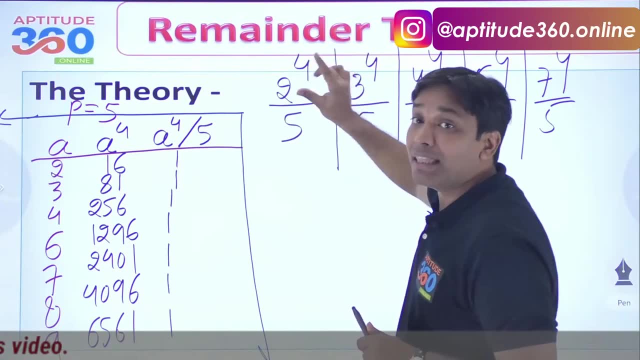 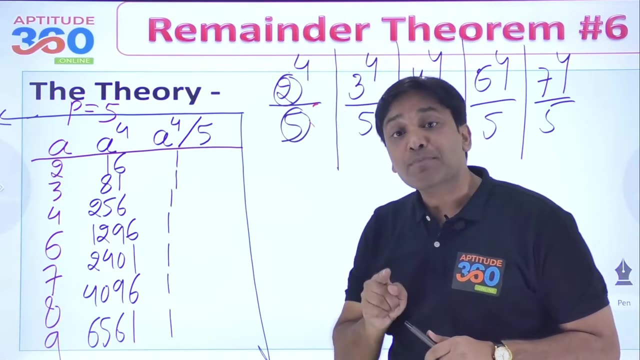 also divide four to power, 4 to five of your mind, then only one will come down. What is the condition? here will have to be a prime number and in the power it has to be one less than that prime number. and condition number three: ye dono number, ye dono number, kya hone chahiye apasme co-prime. 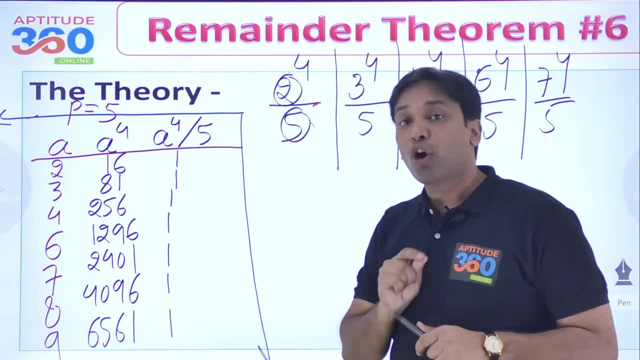 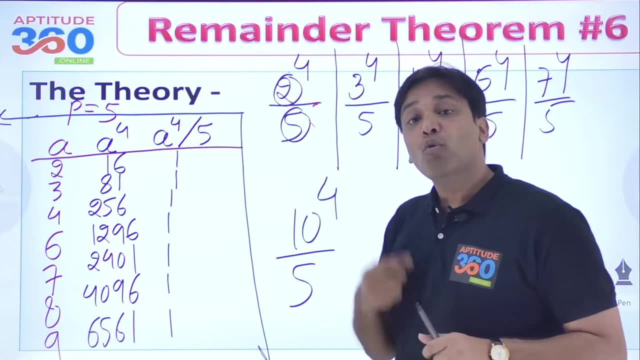 hone chahiye. yaani ki inke beechme koi bhi factor common nahi ho sakta. is that okay? jase, agar mai bol, do 10 divided by 5, can i say, this will give you one as a remainder? no, it is not gonna give. 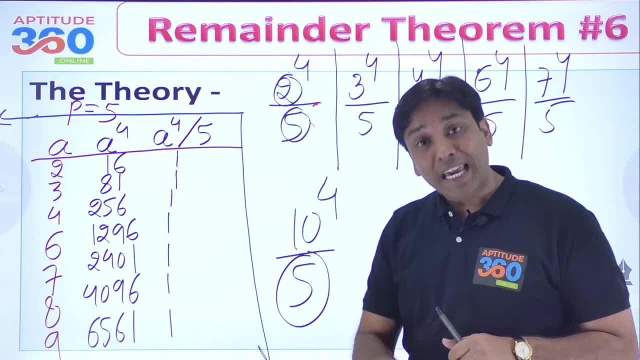 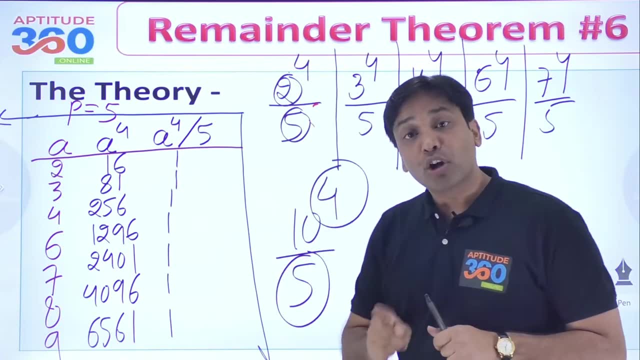 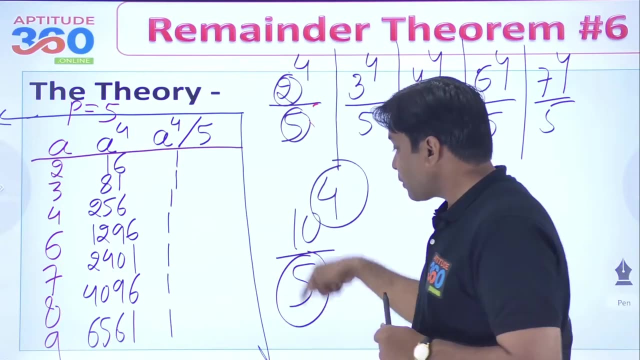 you one as a remainder, because even though, even though this 5 is a prime number, even though in power you have got 5 minus 1, which is 4, but then 10 and 5, both of them are not co-prime numbers. agar ye dono co-prime hote to inke beech ka factor, kya hota sirf 1 common hota, but yahape to 5 dono. 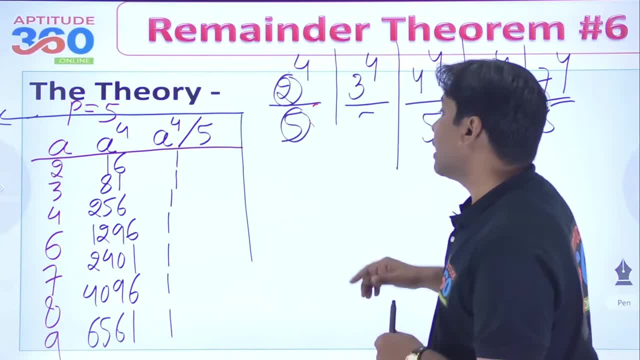 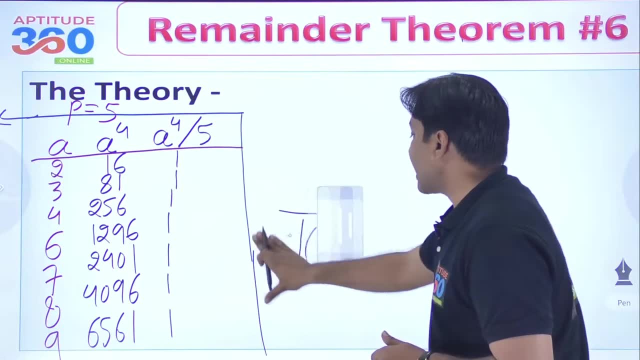 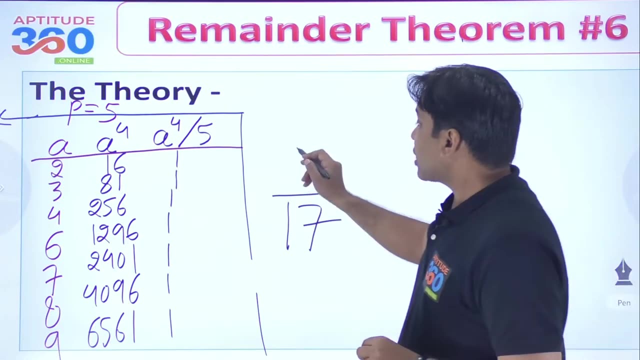 me common hai, isn't it? now, if you understand this thing, can i say this: i am just taking random numbers. i am just taking random numbers. i have got 60, uh 16. i cannot take in the denominator. i can take 17 in the denominator. is 17 a prime number? yes, so i would say that any number, any 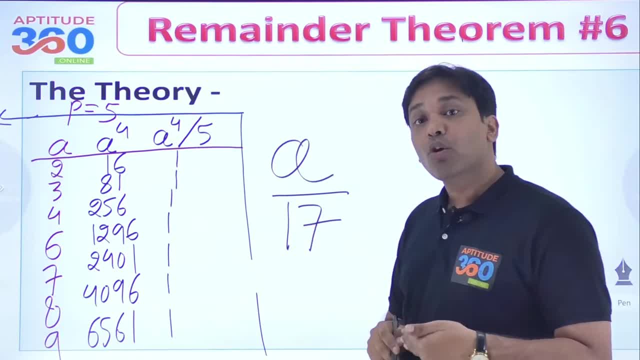 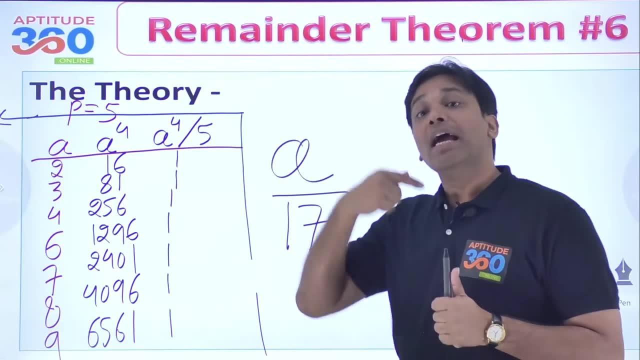 number which is going to be co-prime to which is going to be co-prime to 17 yaani ki a aur 17 ke beechme koi bhi factor common nahi hona chahiye. is tariko ko aur bhi bola ja sakta hai ki a should. 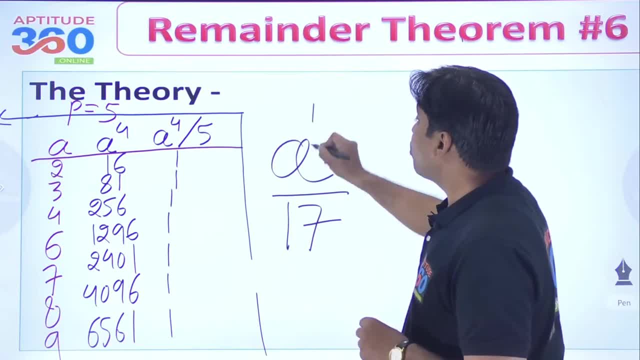 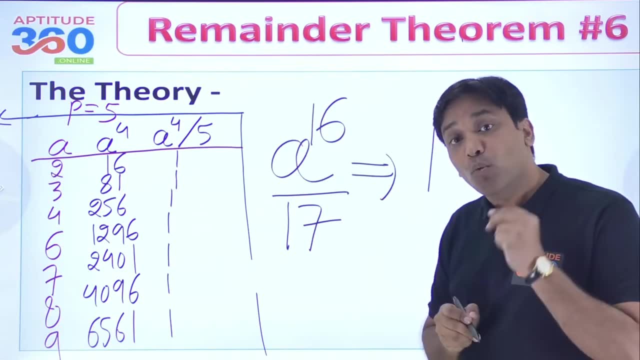 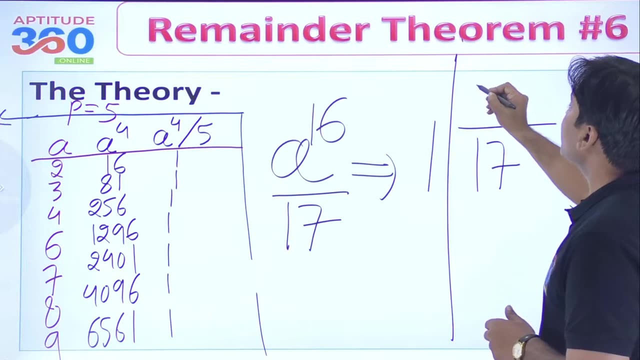 never, ever be multiple of 17, aur agar aisa hua to this n minus 1, ye jo remainder hoga ye hamesha hi 1 aega. one more thing, jaise maine, kya bola this is divided by this and and what if i? 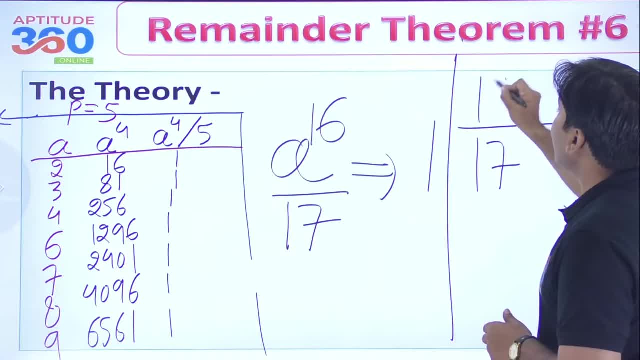 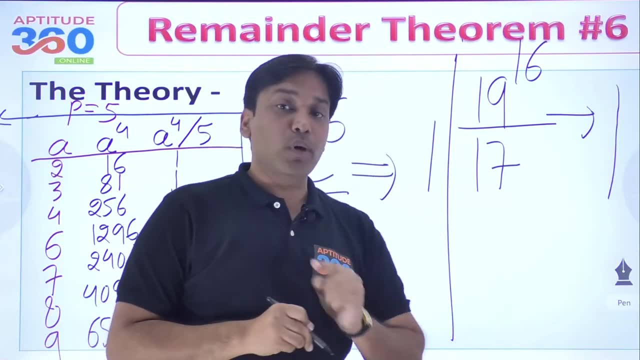 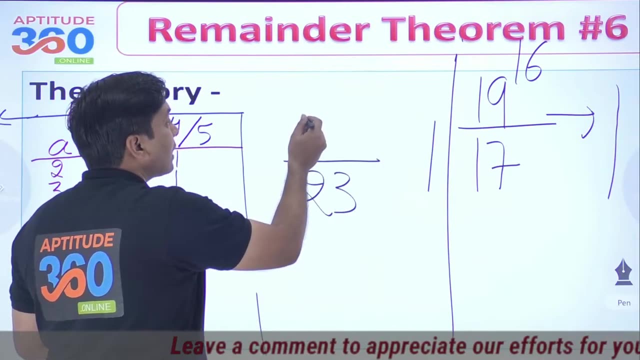 take that number as maybe say 19 is to power 16, will this, will this remainder be 1? yes, that remainder is going to be necessarily 1. if i have got, if i have got 23, if i have got 23, and this over here is 26, is 26. 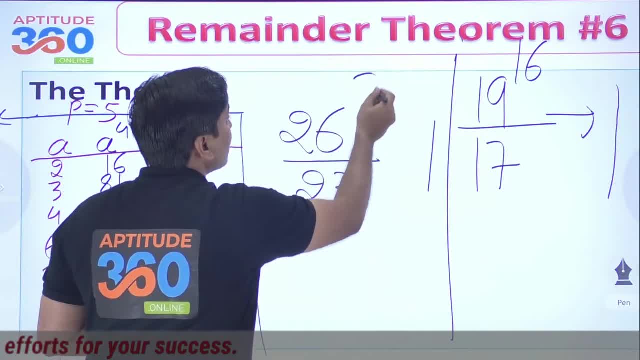 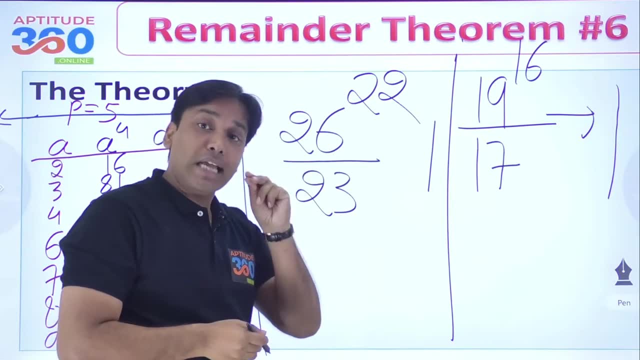 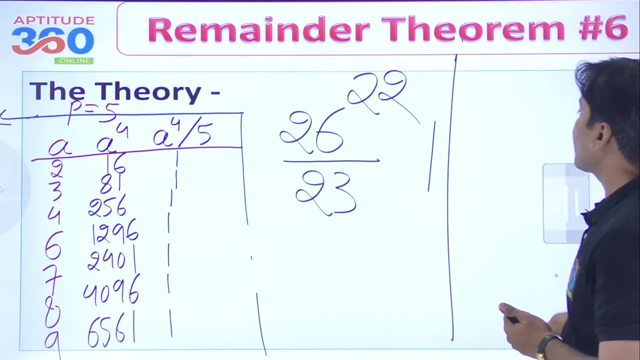 co-prime to 23. yes, so can i say that this is to power: 22 n minus 1. will this give you 1 as a remainder? it is going to give you 1 as a remainder. that is guaranteed. that is what fermat little theorem is all about. right, agar, agar, yaha pe kuch aisa de diya jaye aapko. 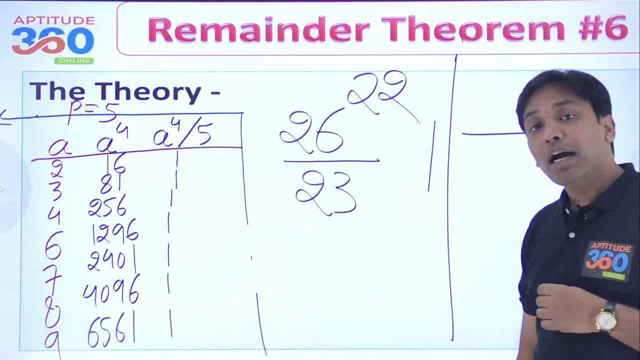 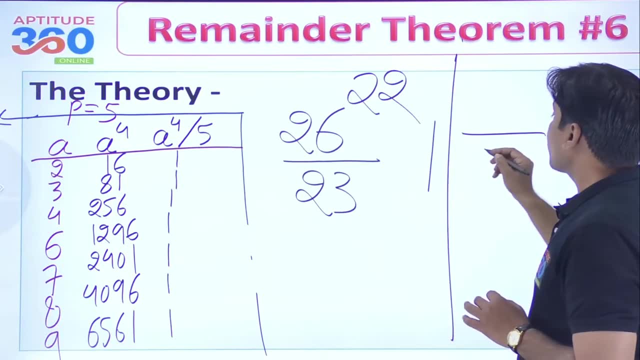 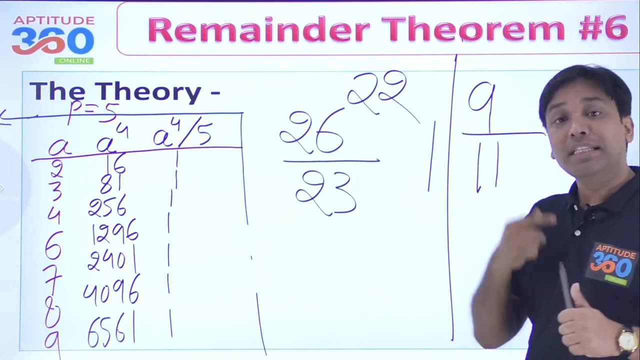 denominator, denominator me hamesha hi kya hoga? it will have to be, it will have to be a prime number, aur kuch bhi nahi ho sakta, jaise maine yaha pe le liya. say, for example: divide kar diya 11 se and yaha pe rakh diya 9 right is 9 a co-prime to 11. yes to 9 is. 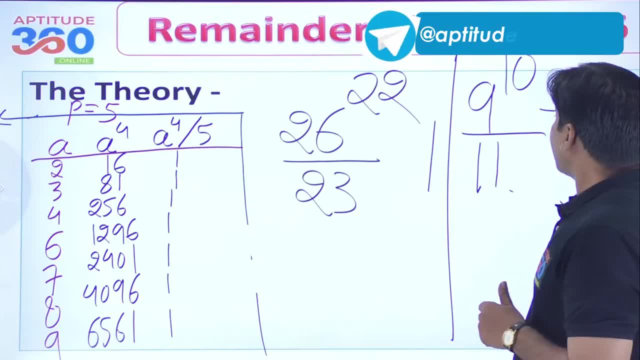 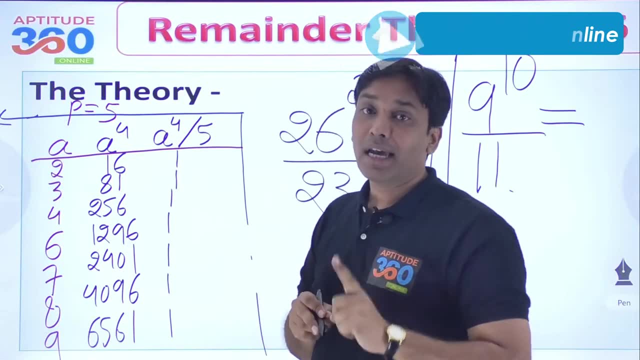 to power 10, which is which is 11 minus 1. agar aapne 9 is to power 10, ko 11, se divide kya to remainder? kya aega? 1 hi aega. i hope everybody is understanding this entire thing. this is: 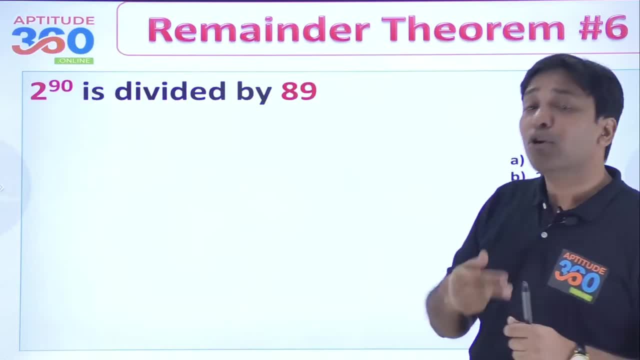 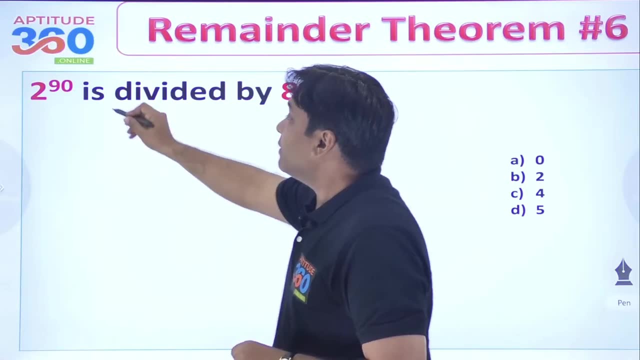 very, very, very simple right chalo, agar aapko ye cheez samajh mein aati hai to. we will be utilizing those concepts over here in the in the problem solving. the first problem out here is: what, if? what? if 2 is to power, 90 is getting divided by. 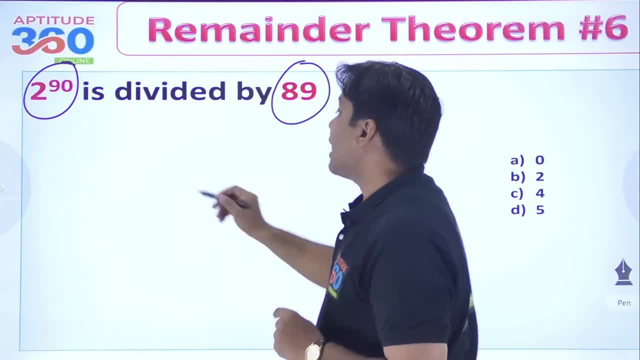 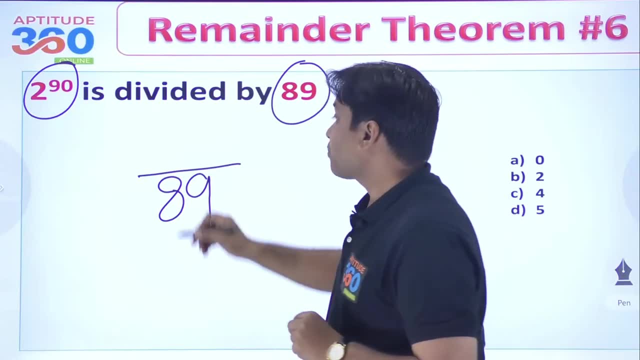 2 is to power 89. what is going to be the remainder? abab dhyan se samajh mein hai. is 89 a prime number? yes, it is a prime number. and then you have got 2. is 2 co-prime to 89? yes, 2 is co-prime. 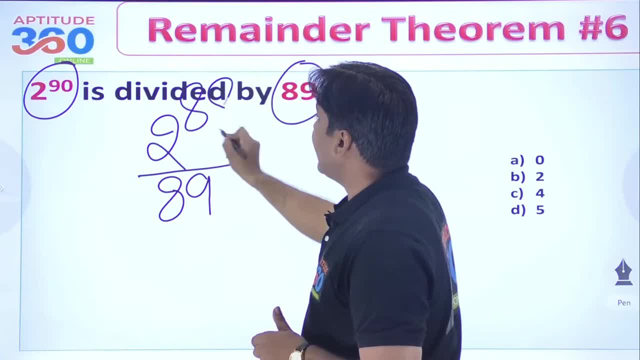 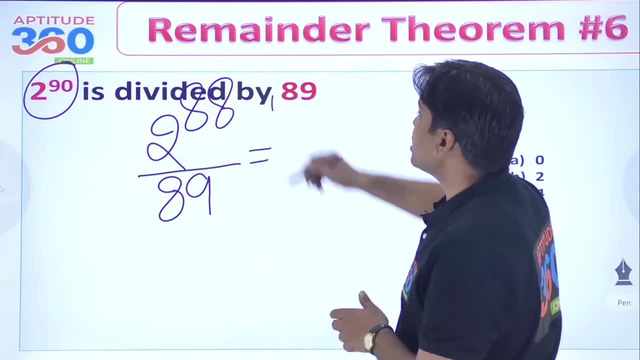 to 89, and can i say that this is to power. 88 will give you 1 as a remainder. will this be 1 as a remainder? aek sa cheez, yeh samajh mein aani chahiye, dosri cheez wo hamare ko. 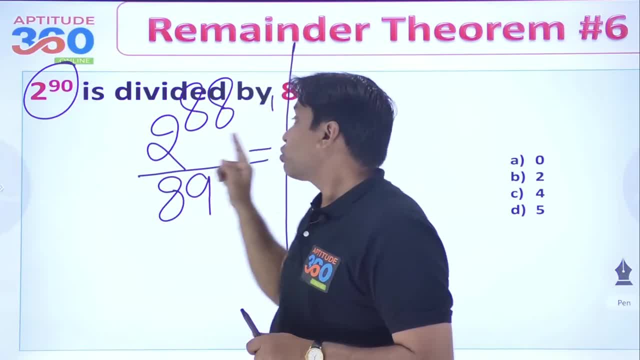 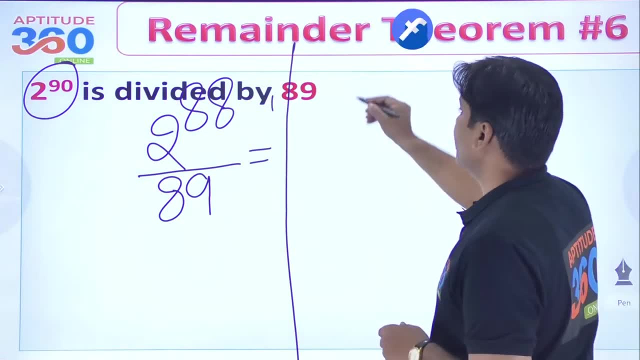 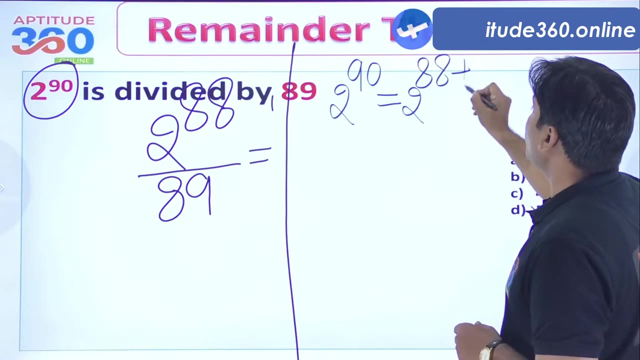 kya dekhe rakha ho hai. problem mein, they have not given us 2 is to power 88. rather, they have given us 2 is to power, 2 is to power 90. so what i should be doing here is i should be writing this: two is to power 90 as 2 is to power 88 plus 2, right, and then you can. 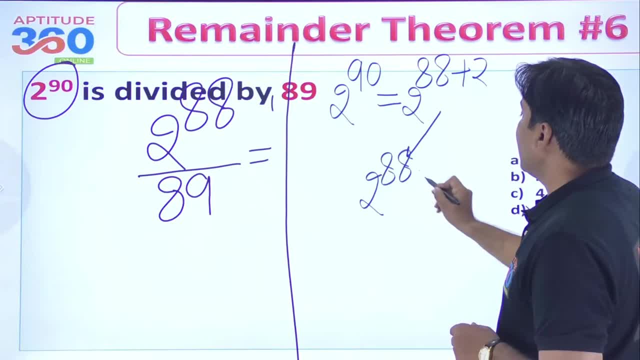 simplify this and you can say that this is 2 is to power 88, into into 2 is to power 2, which is nothing but 4, right, alright, is nothing but four. and if you divide this number by 89, what is going to happen now? what is going? 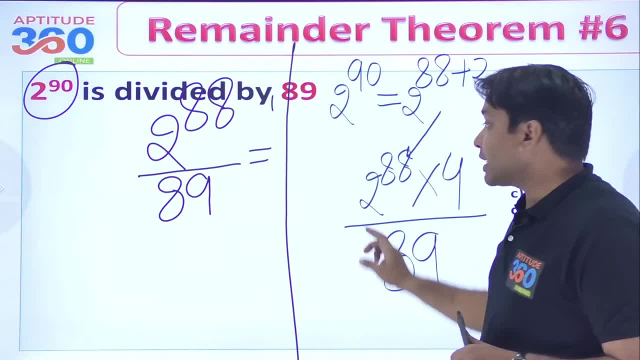 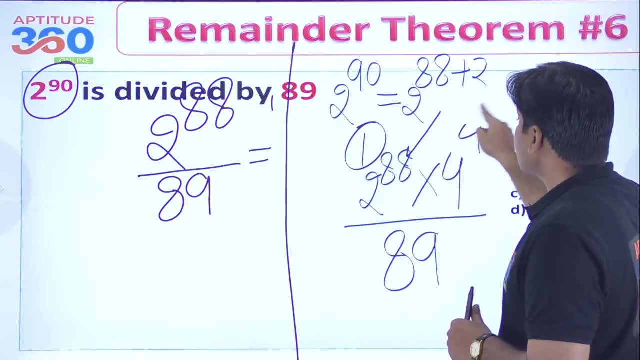 to happen now. if 2 is to power 88 is getting divided by 81- 89, this remainder comes out as 1. if 4 is getting divided by 89, this remainder is coming out as 4. because these two numbers, these two numbers, this is what we have been learning since video number one of the remainder? 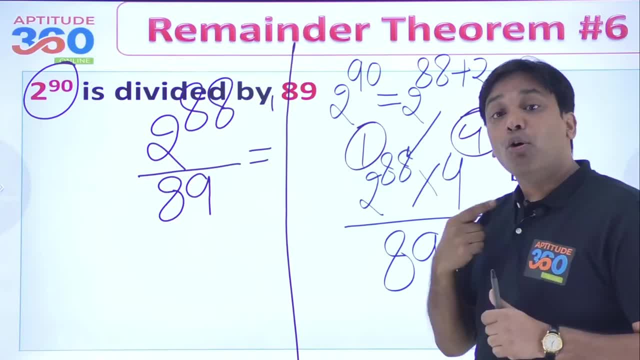 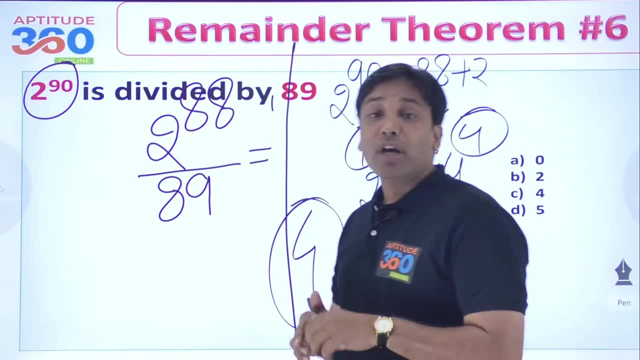 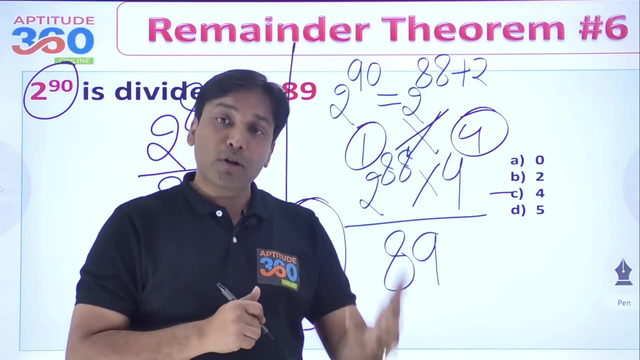 theorem that if these two numbers are getting multiplied, then what does this mean? that these remainders will also get multiplied and their answer will be 4, and that is what will be your answer. is that okay? so if you have not seen that video, number one, where we talked about the basics, 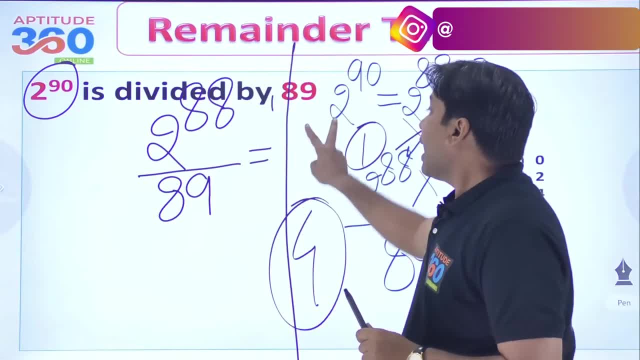 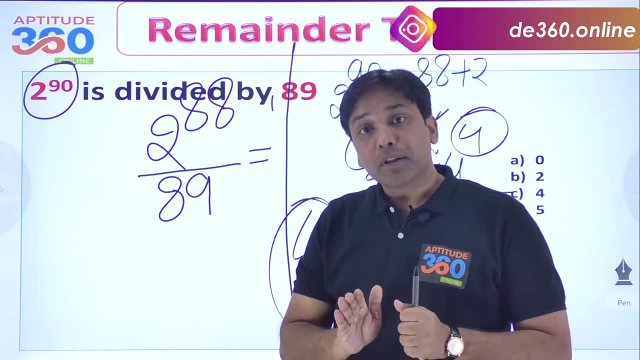 please go and watch that one right now. having said that, you see how simplified the work has become. toast power: 90 upon 89. it is so, so, so simple. it is just that you will have to understand this little theorem. its little theorem is actually very little to understand. 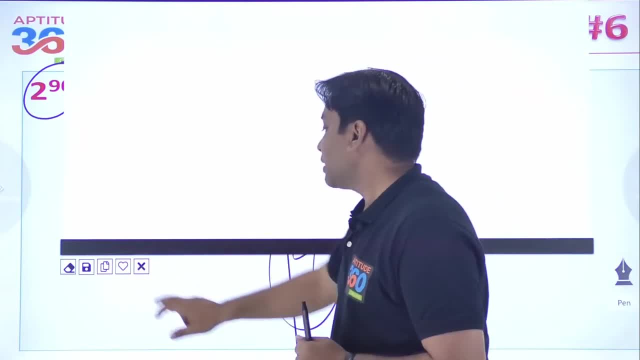 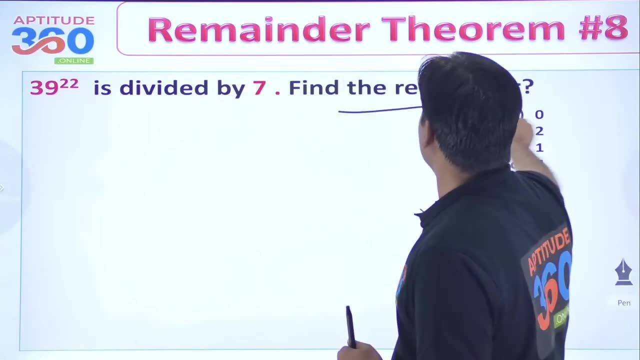 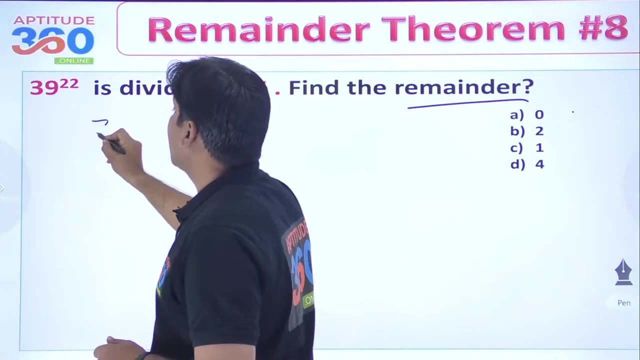 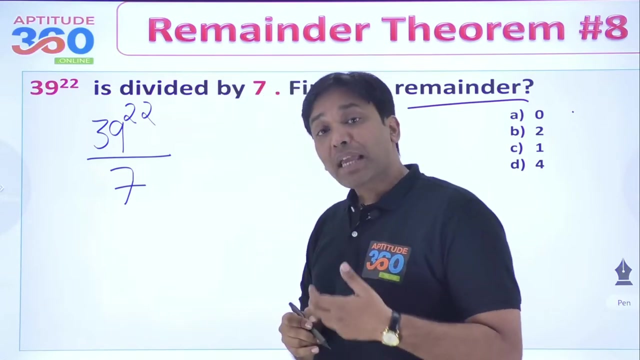 now. now, what if? what if we solve the next problem, and this next problem is 3, this number divided by this number, find the remainder. so solve it properly. it is a simple problem to solve. can I say that 39 is to power 22 divided by 7, is 7 a prime number? 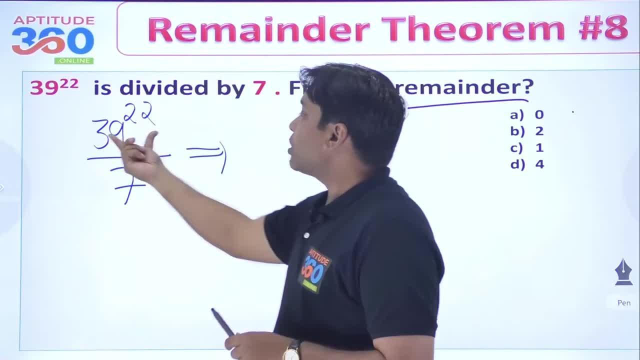 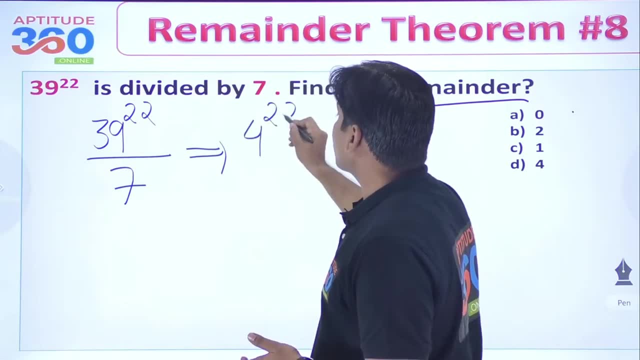 yes, 7, we can. we can simplify this. you know what. what we can do is: if 39 is getting divided by 7, will the remainder be 4. so can we write this problem as 4 is to power. 22 divided by 7 is that. 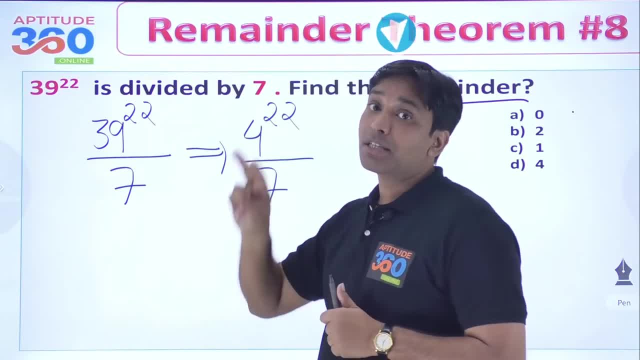 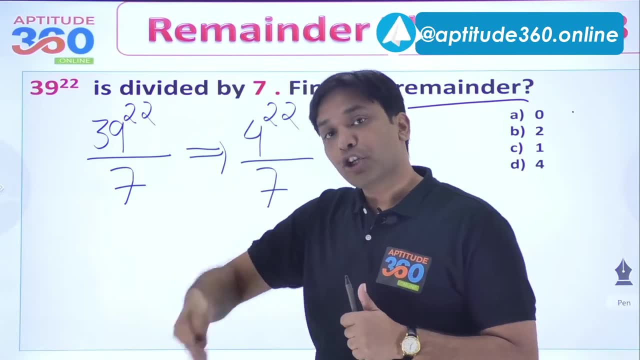 okay, now everybody understands this thing. this is what we discussed in video number 2 of this series. if we divide 39 by 7, then what remainder will come? 4 into 4, into 4 into 4. how many times? this is going to be 22 times. so what did I write? 4 is to power, 22 divided by 7. now I am going to use 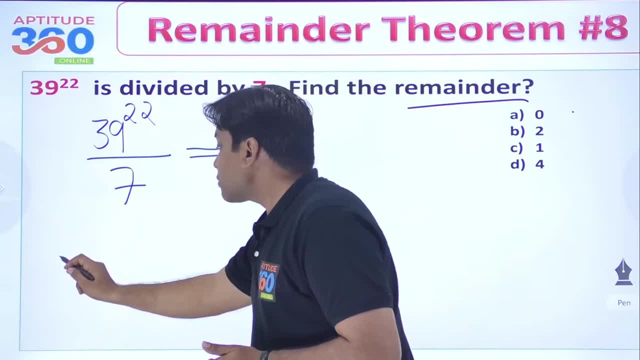 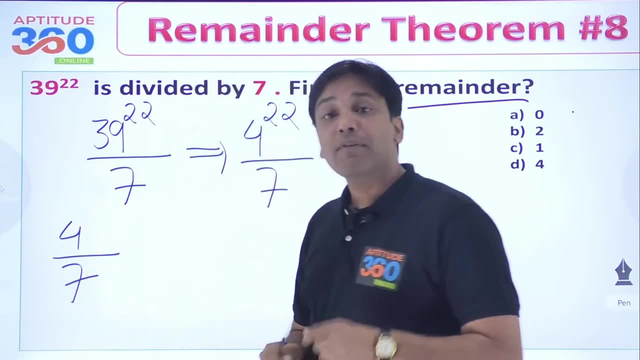 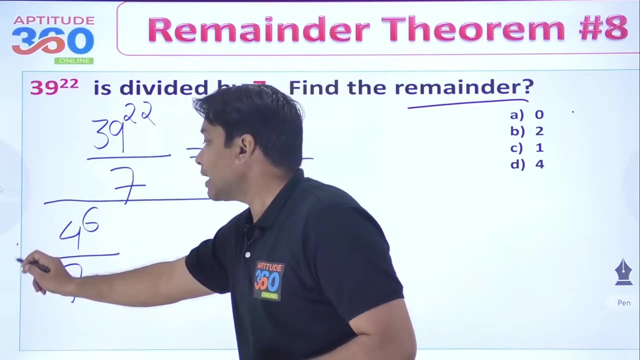 that little theorem, Fermat's little theorem, and I would say that, I would say that 7 is in the denominator. 7 is being divided and this number is 4, 4 and 7. both of them are co-prime to each other. so what I will write here, this number means, if I take out the remainder here, if I take out this: 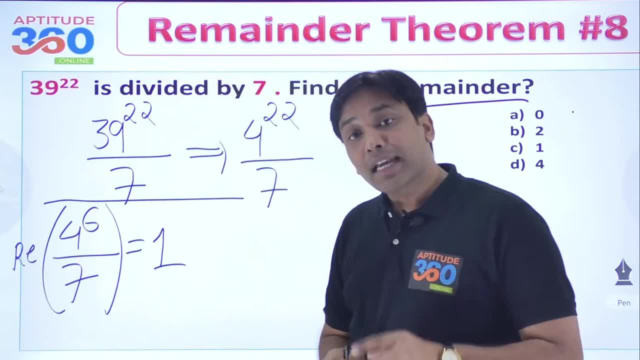 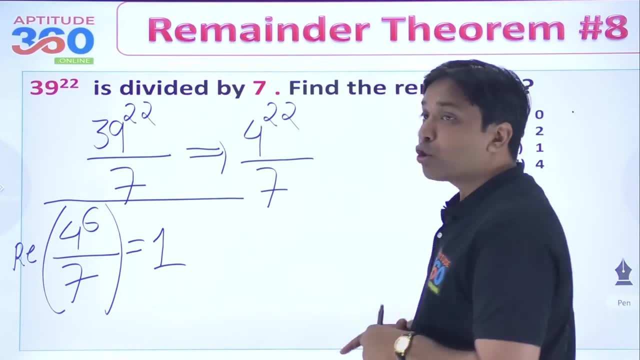 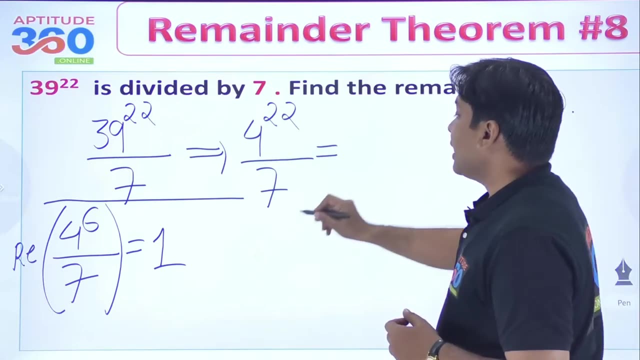 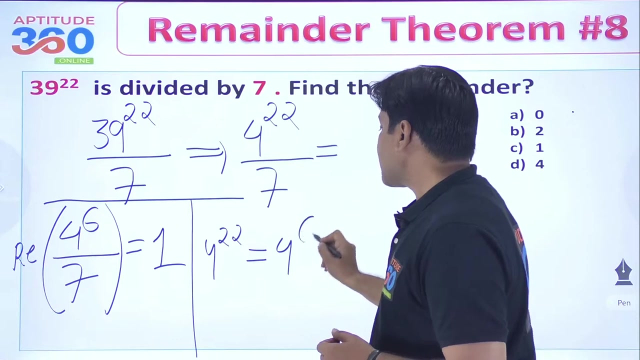 remainder, then this remainder will necessarily come out to be 1. is that okay? and but how much is given here? it is given here so 22. so what is that we should be doing first? we take this to this so that we can simplify it more. so can I say? can I say 4 is to power? 22 can be written as 4 is to power, 6 into 3 plus 4. 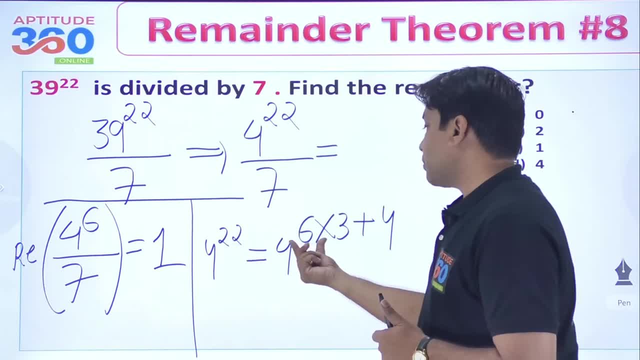 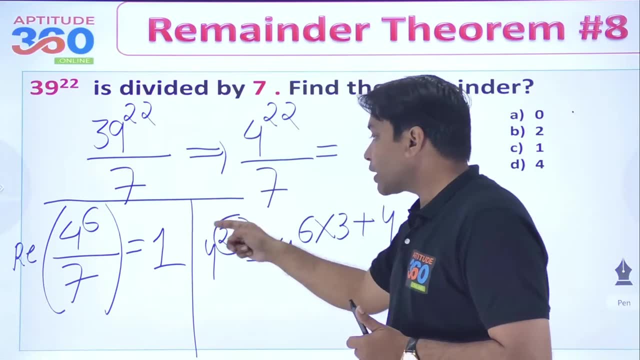 simple. it is: 4 is to power. 22 can be written as: 4 is to power. 6 into 3 plus 6 into 3 is 18, 18 plus 4 is 22. what will we do? we will divide this 22 by 4. sorry, this 22. 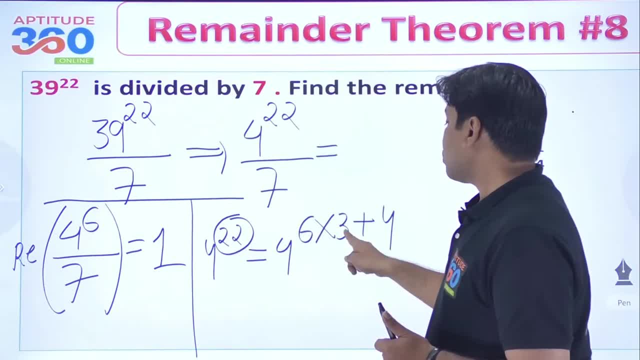 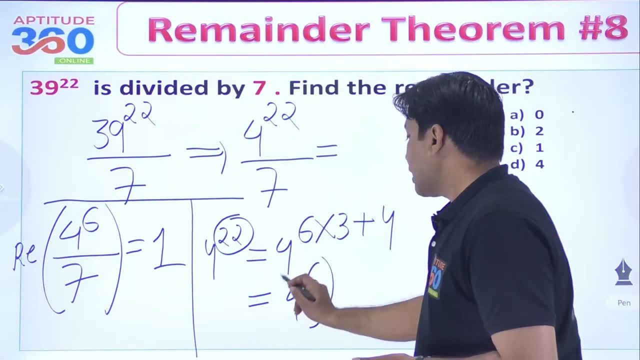 we will divide 22 by 6. if we divide 22 by 6, then 3 will be quotient and 4 will be remainder. now what will you do? write it like this: 4 is to power, 6 is to power. 3 into this number is 4 is to power 4. 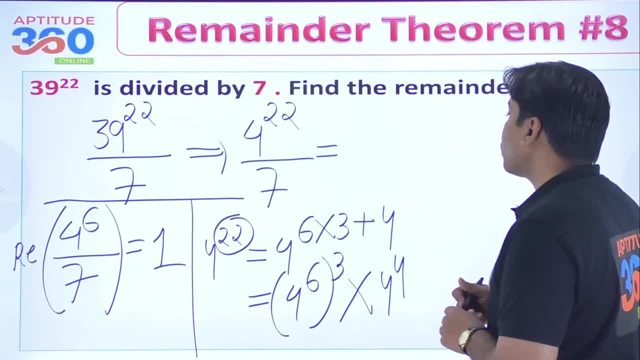 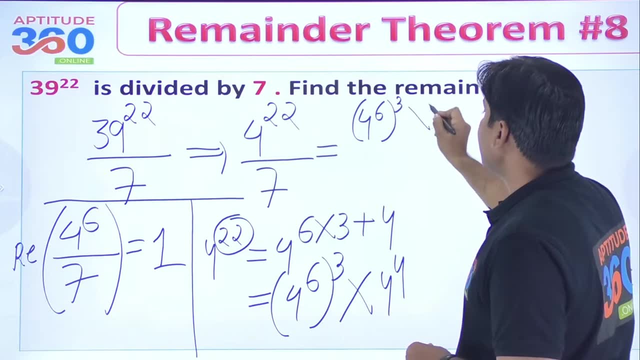 is that ok? now what is that you should be doing? this number is 4 is to power 6 into 3, and this number is 4 is to power 4. what can we write? 4 is to power 4, 16 into 16. 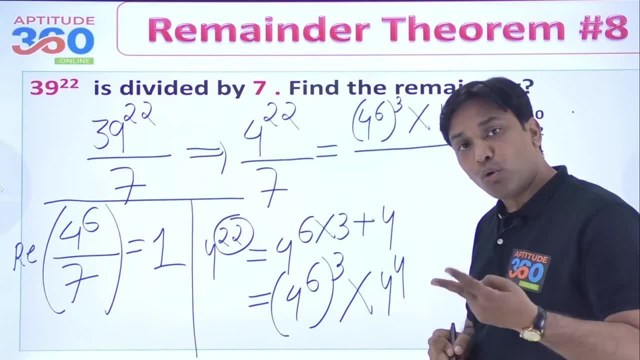 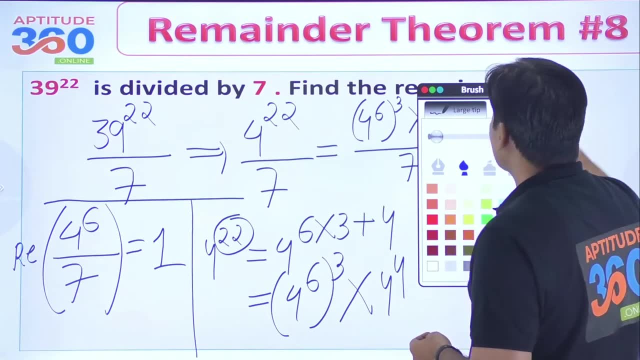 4 is to power, 4 is 4 is to power 2 into 4 is to power 2 and divide it by 7. now you see how easy the problem will be. now try to understand this. 4 is to power 6 divided by 7. 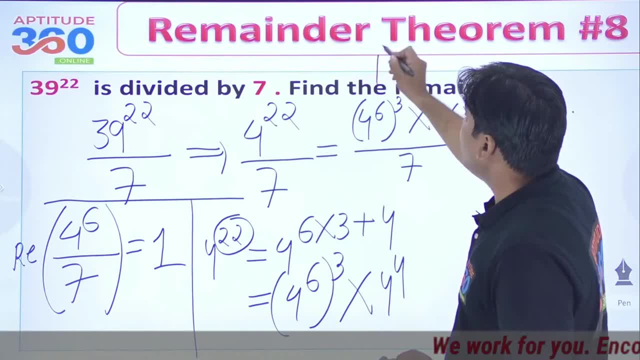 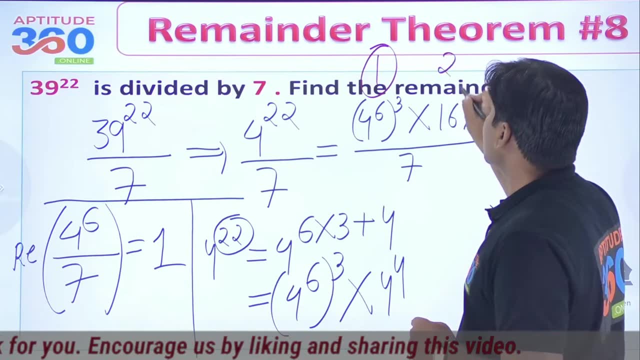 the fermus laden theorem says that the remainder is 1, and if it is in the power of 3 over here, this remainder will be 1. if 16 is getting divided by 7, what is the remainder? this remainder is 2 if this 16 is getting divided by 7. 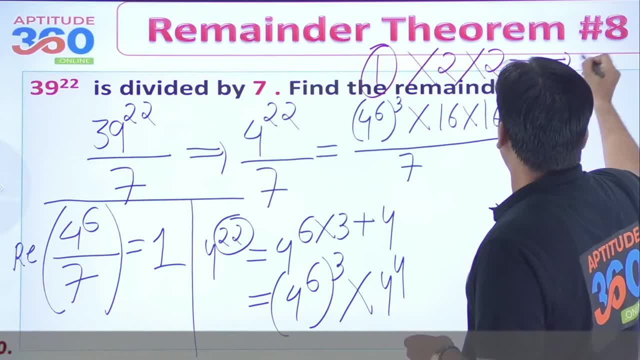 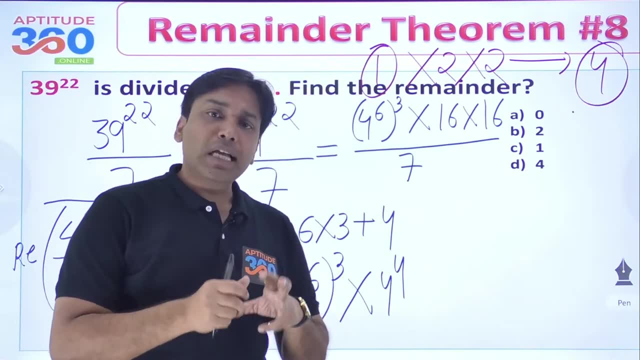 this remainder is 2, because these numbers are getting multiplied. what is going to be the remainder? this remainder is going to be 4. fermus laden theorem will be applied and we will do some adjustment. the problem will come out by itself, so we don't have to get disheartened. 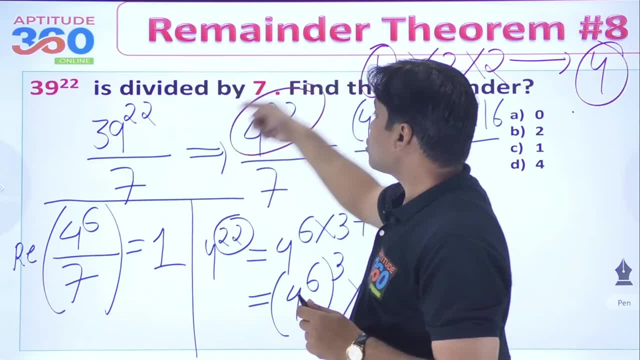 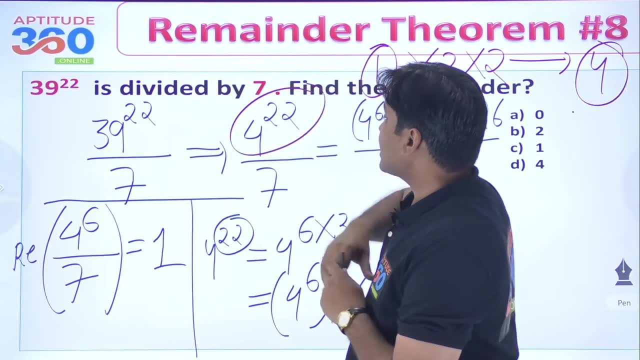 when they have given us. when they have given us, 4 is to power 22, which is not the multiple of 6. had it been the multiple of 6, then the problem would have been very easy, like if you were asked. if you were asked, 4 is to power 30. 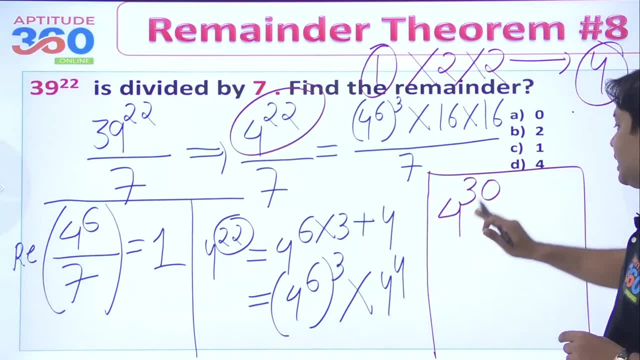 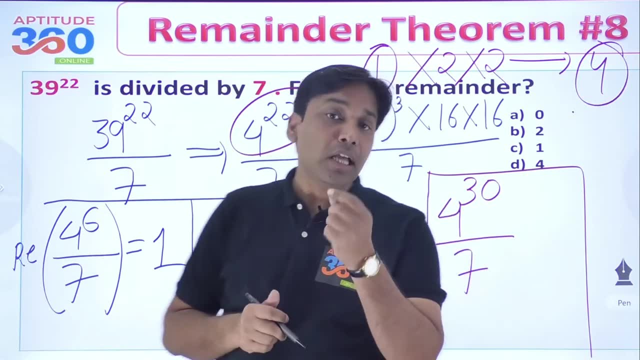 4 is to power 30. 4 is to power 30 divided by 7. so what is going to be the remainder? 4 is to power 30 divided by 7. now this remainder necessarily will be 1. why this is going to be 1. 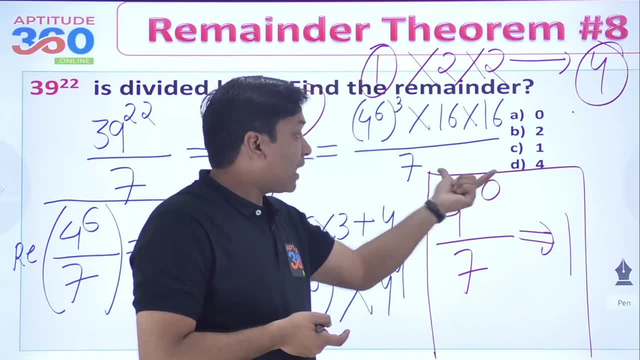 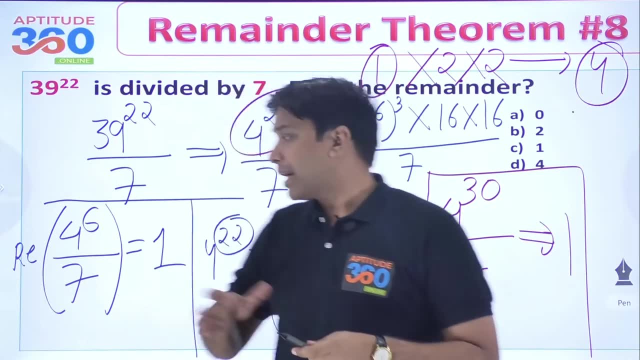 because 4 is to power, 6 should give you 1 as a remainder, and 30 is what? 6 into 5. hence the remainder will be coming out as 1, but if it is not the multiple, then we will do some adjustment, like we have given. 4 is to power 22. 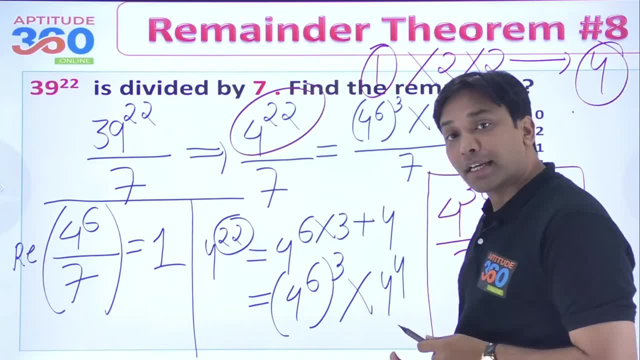 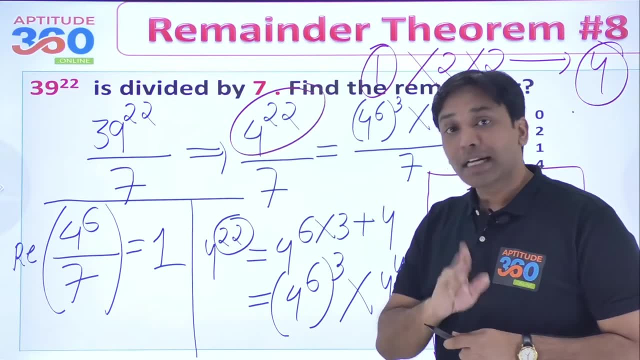 so what we will do for 4 is to power 22. we will do 16 to the power 3 plus 4 which is common, which will not come in the multiple. we will keep it separately and that only will be a big remainder. that has to be the understanding. 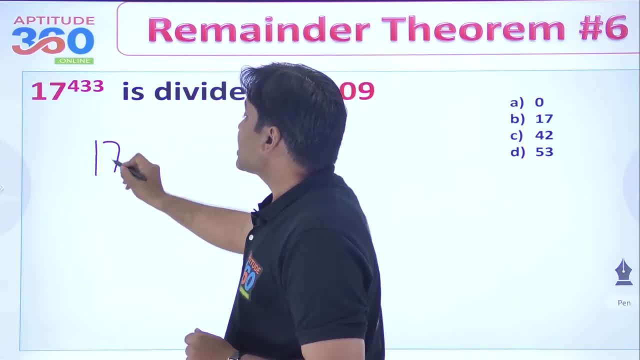 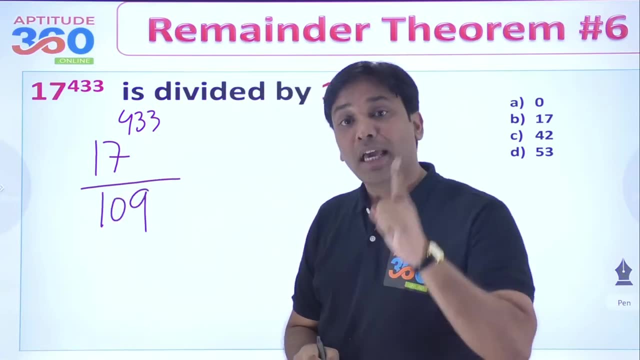 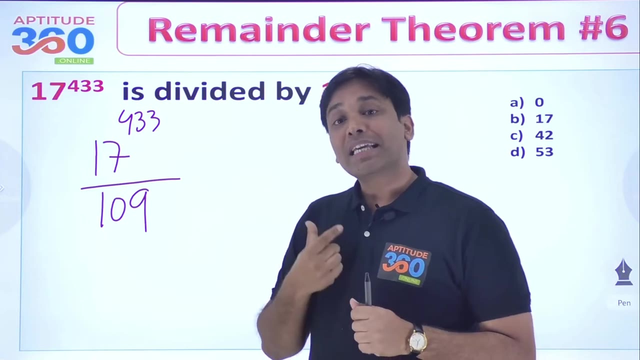 so, if you understand this thing, I am going to solve this problem now. see this: this says 17 is to power 433 divided by 10109. the question number 1 is 109, a prime number. if you do not know how to determine whether a given number 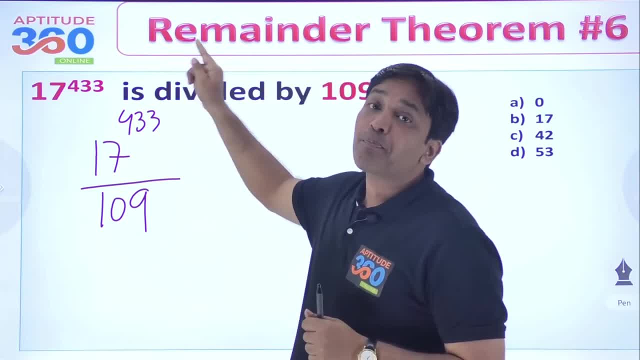 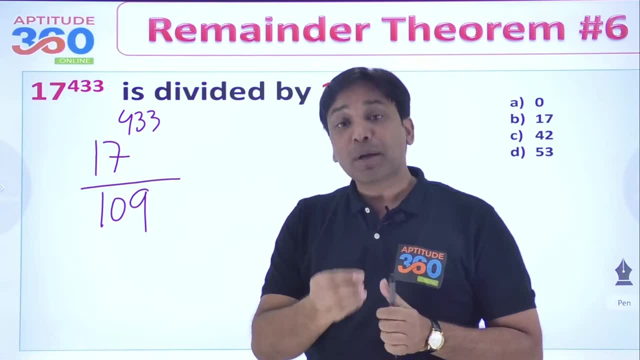 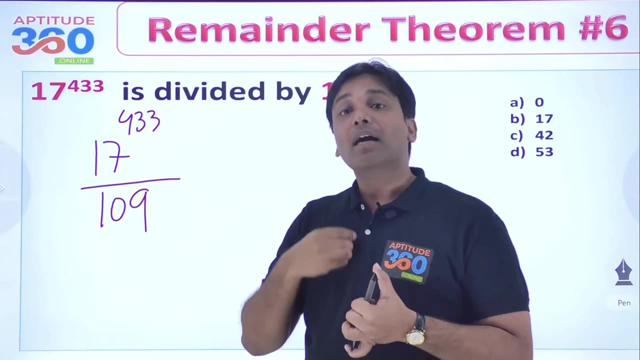 is prime or not. you need to go in this video and see as to how you can find out whether a given number is a prime number or not, because this concept is used in many places. no one knows what is the number. is it prime or composite, or what is it? 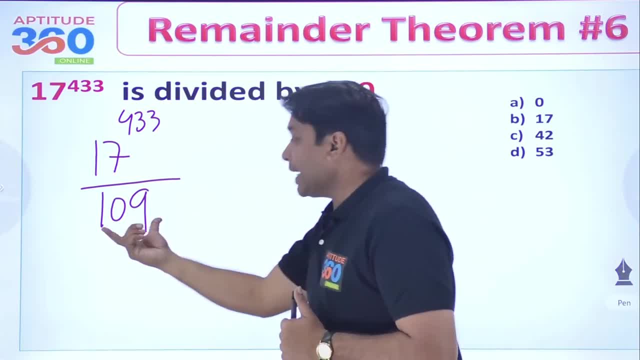 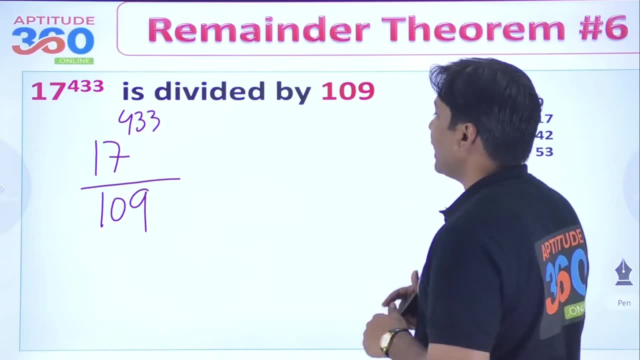 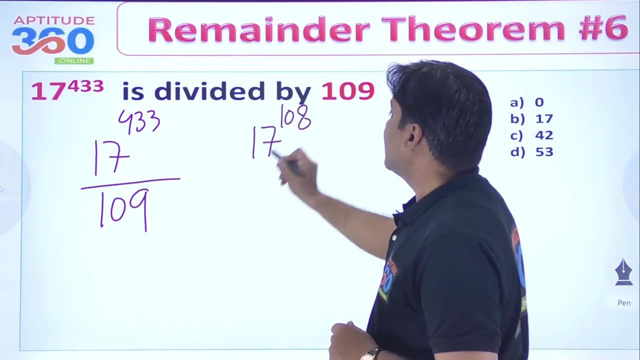 and there are many problems in examination scenario. so I say that 109 is a prime number and there is no common factor between 17 and 109. so I would say this: I would say that 17 is to power 108 divided by 109. the remainder of this. 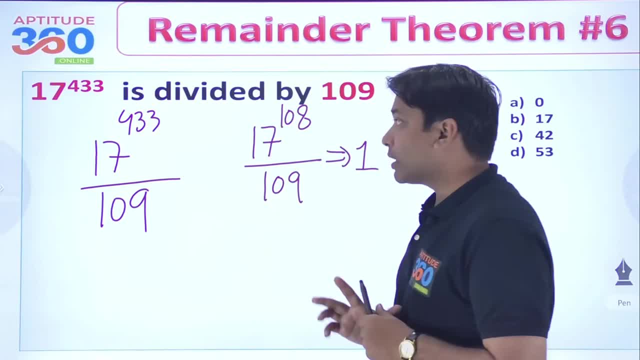 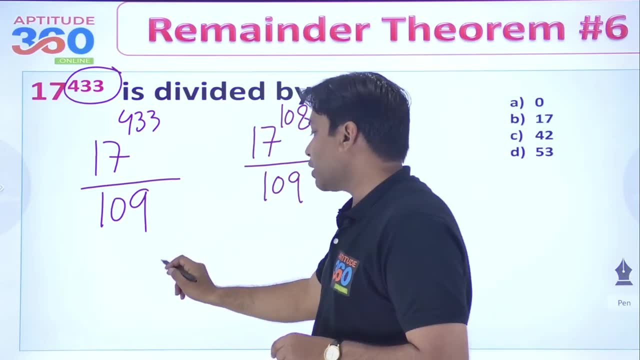 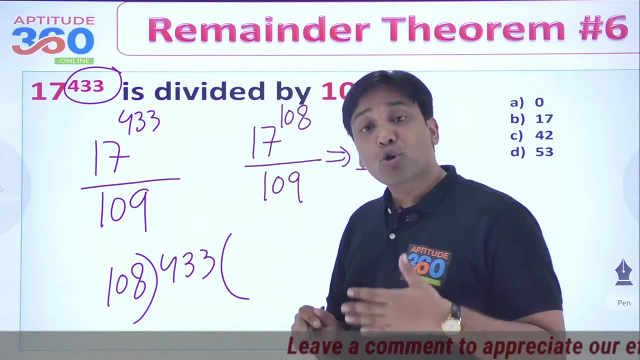 will be 1. is that ok? now what is given to you? 433. divide 433 by 10109, divide it by 108, and if you divide it by 108, how many times will it go? it will be 432. that remainder will be 1. 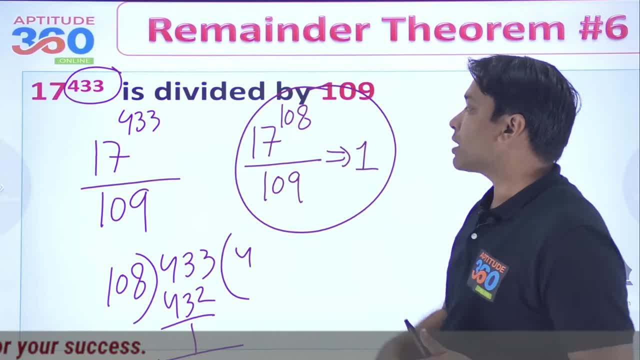 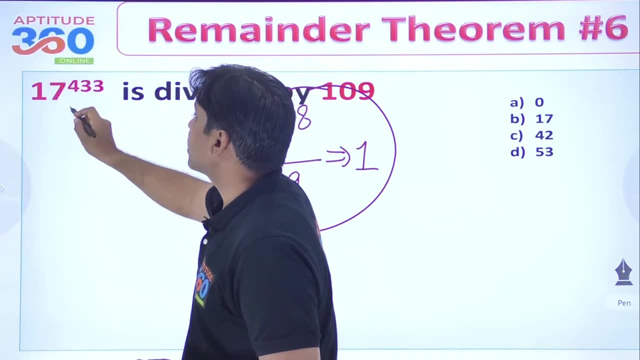 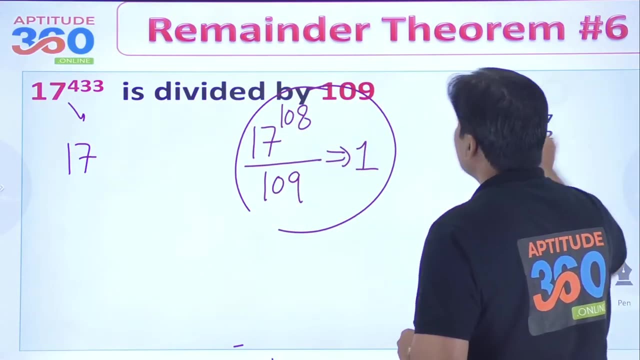 so what I will do is- because I know that this is how it is going to look like- how will I write this number? I will write this number. this number is 17 is to power. now. see this one very carefully, see this one very carefully. this is going to be what 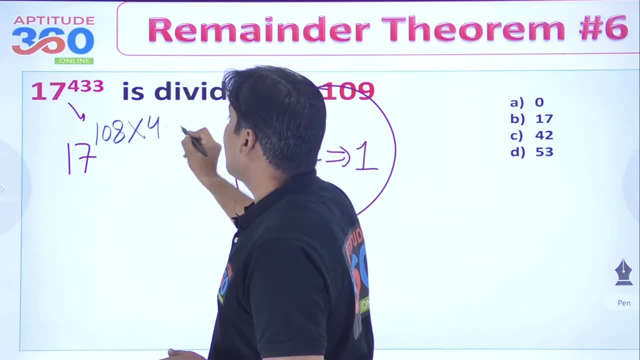 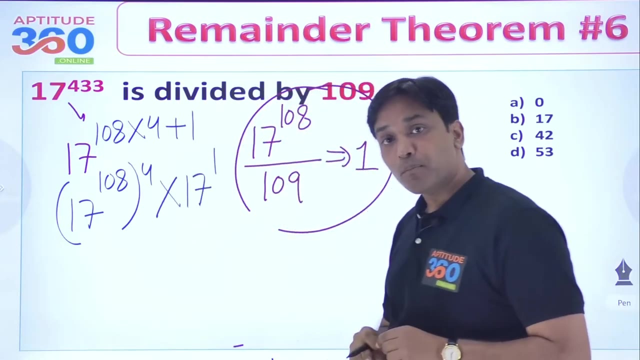 108 into 4 plus 1, then we can write this number as: 7 is to power 108, this is to power. 4 into 17 is to power 1. is that ok? now we know for sure that if I am going to divide this number by, 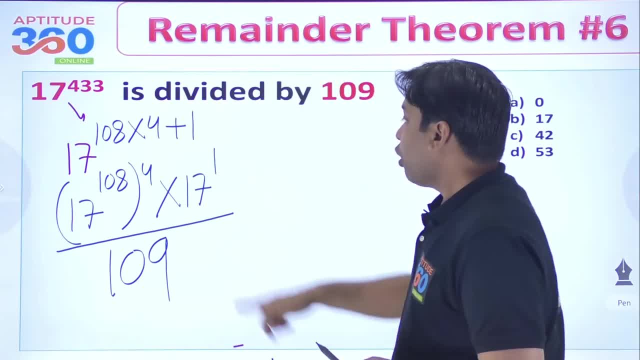 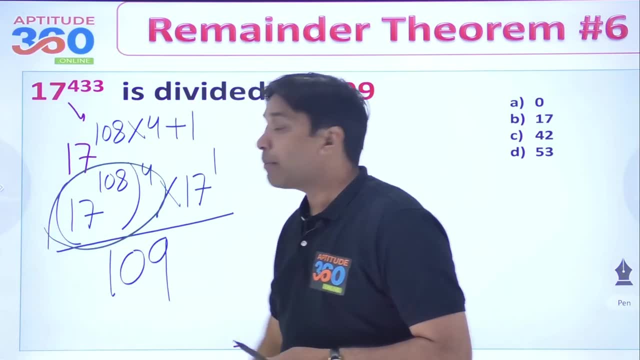 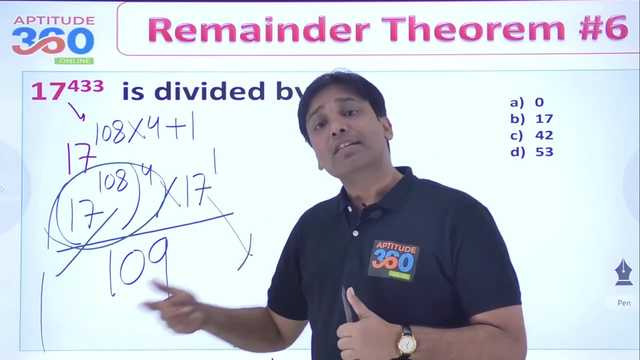 109, 109 over here. I am going to get 1 as a remainder. over here, I will be getting 1 as a remainder. here. this number is going to get me 1 as a remainder. so here the remainder is 1, and because 17 is not being divided by 109, 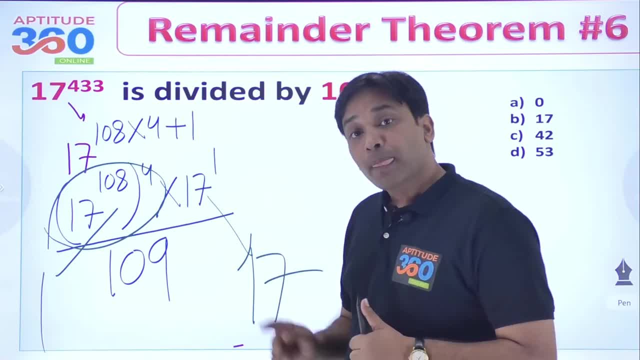 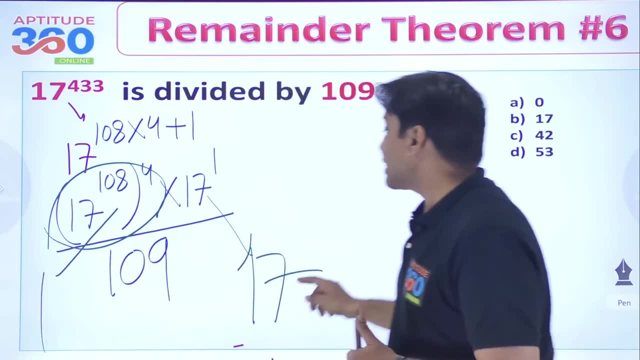 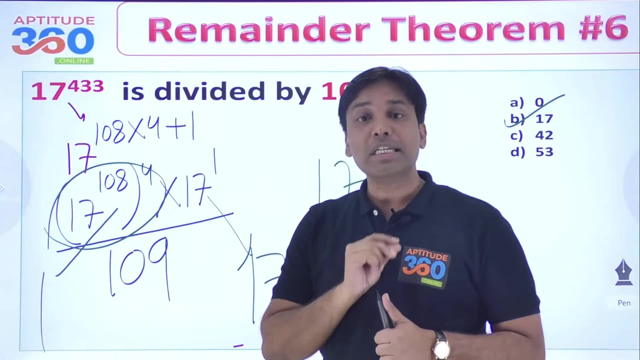 so only 17 will remain as a remainder. so what will be the final remainder? because these two numbers are getting multiplied, remainders are also going to get multiplied 1 into 17. 17 is the answer. this is so, so, so simple. just concentration is needed. 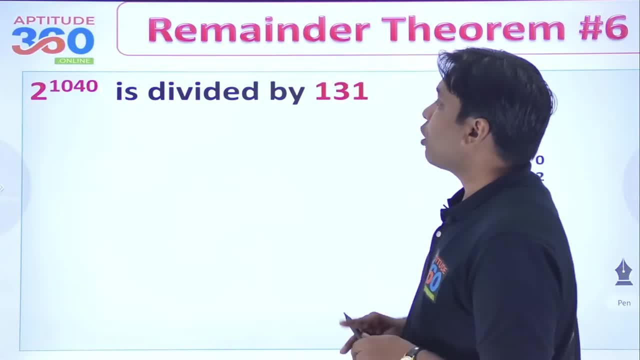 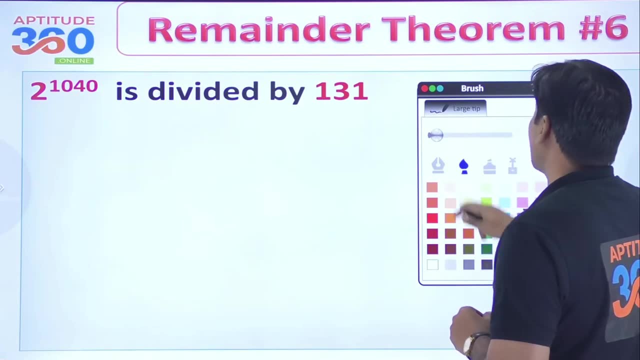 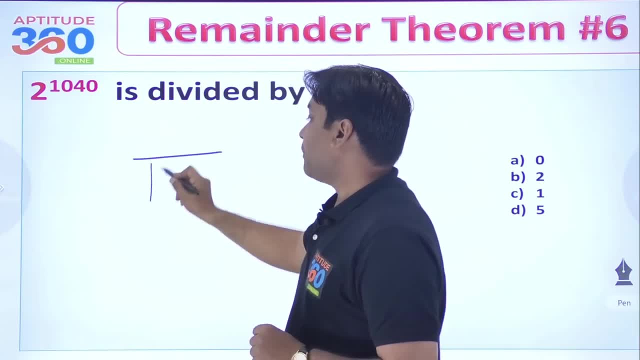 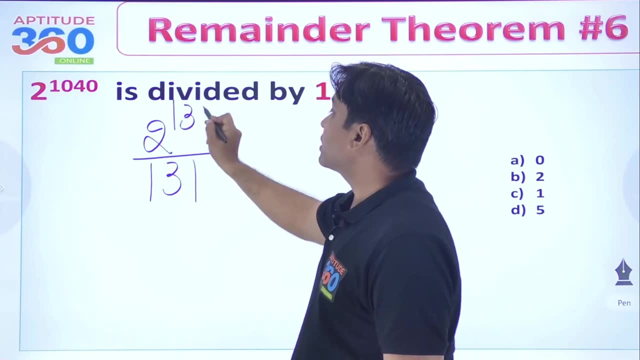 by the time I change the colour of the slide, because if the denominator is 131 and 131 is a prime number, so I would say that 2 is to power 130. if 2 is to power, 130 is getting divided by 131. this remainder. 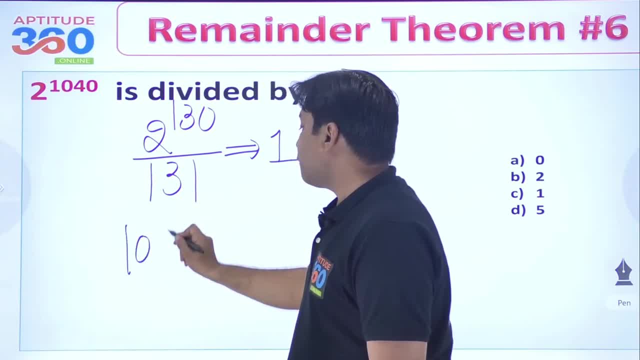 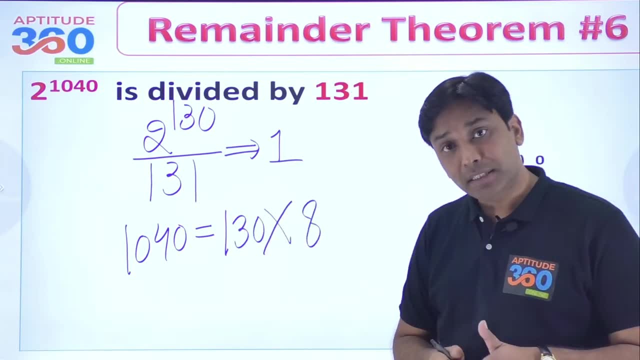 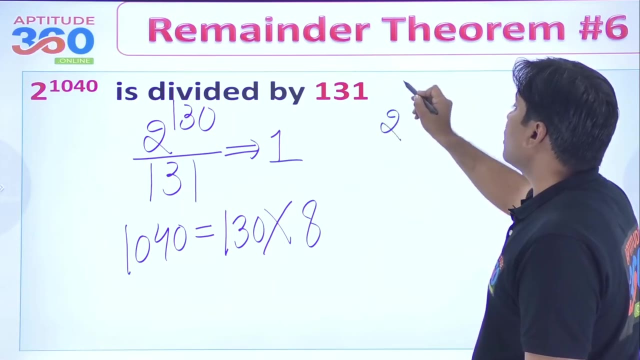 necessarily is going to be 1 and 1040. 1040 is nothing but this number. into this number, into 8, right? so what will happen? how much remainder will come out? 2 is to power. 1040 can be written as 2 is to power. 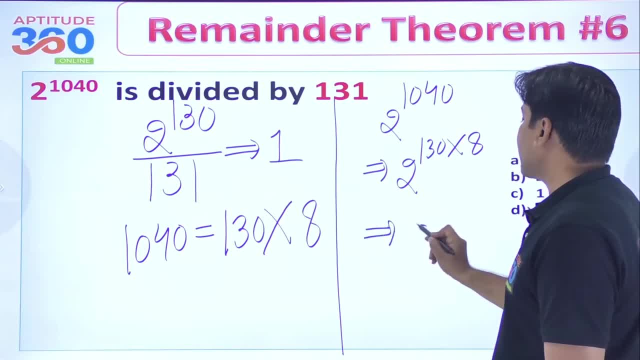 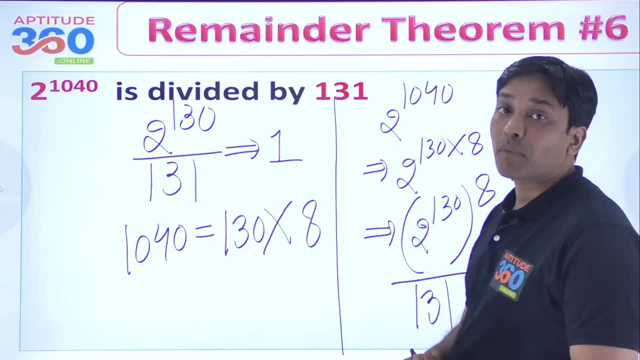 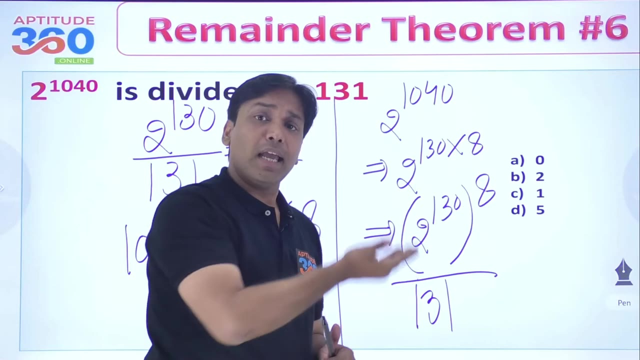 130 into 8, and you know for sure that this is 130, and this entire is to power. 8 divided by 131, 131, this number gets you 1 as a remainder. so what difference does it make? if it is not 8, the remainder that will come out. 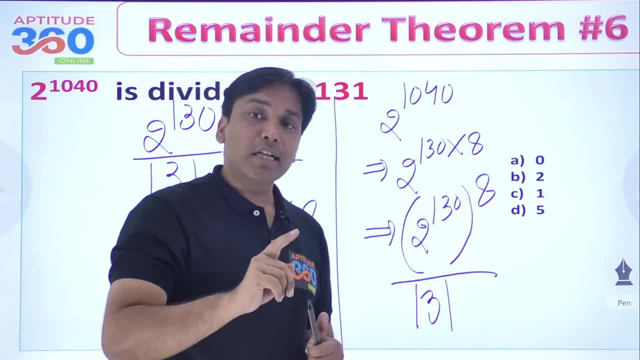 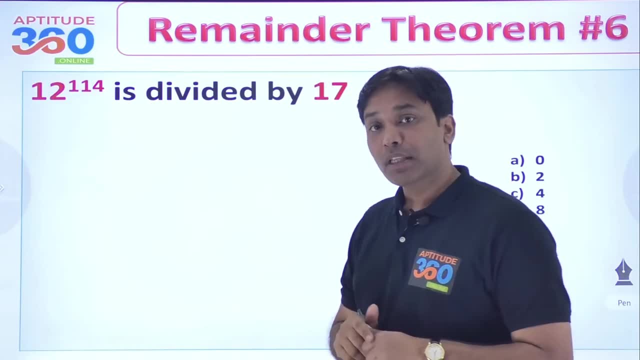 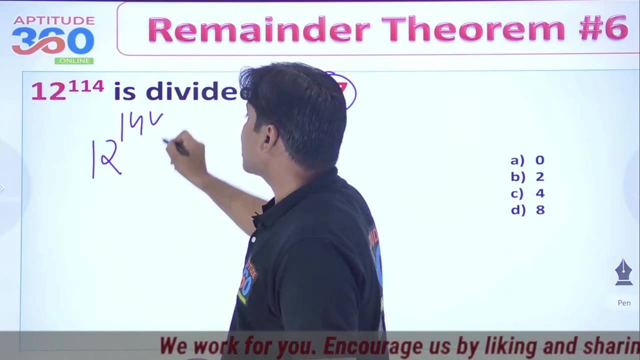 the remainder will also be nothing but 1. is that ok? so answer of this problem is going to be: is going to be 1. how about this one? how about this one? is it a prime number? yes, 17 is a prime number. so 12 is to power 144. 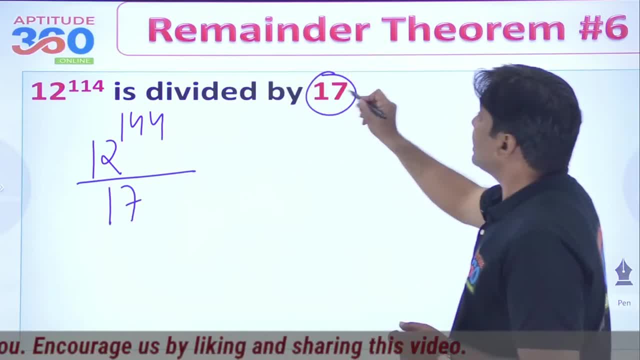 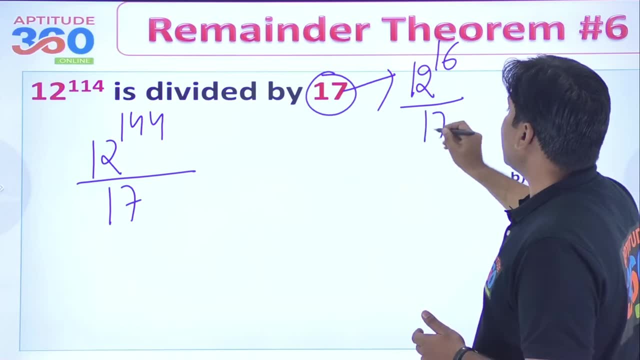 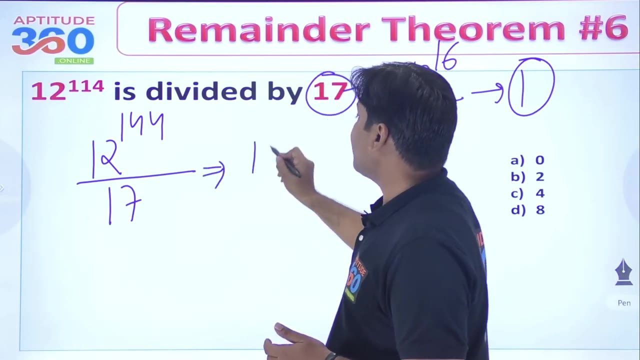 divided by 17 is being asked. what will this theorem say? what will this little theorem say? 12 is to power. 16 divided by 17 certainly is going to give you 1 as a remainder right. so can we say this number as 12 is to power 144. 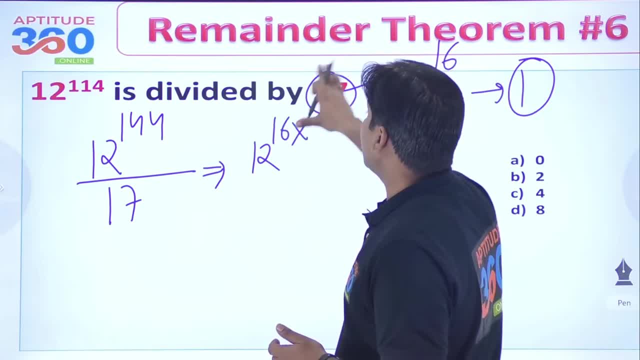 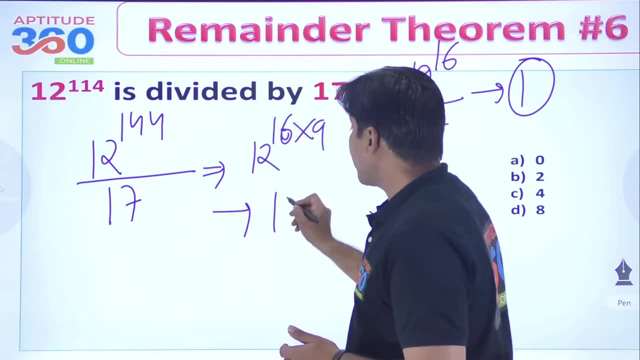 144 can be written as 16 into this, number is 9, and if this is 12 is to power 16 into 9, so we can write: this is 12 is to power 16. sorry, my bad, my bad, 12 is to power 16. 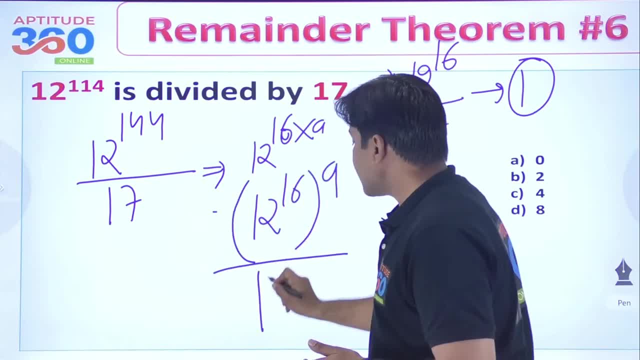 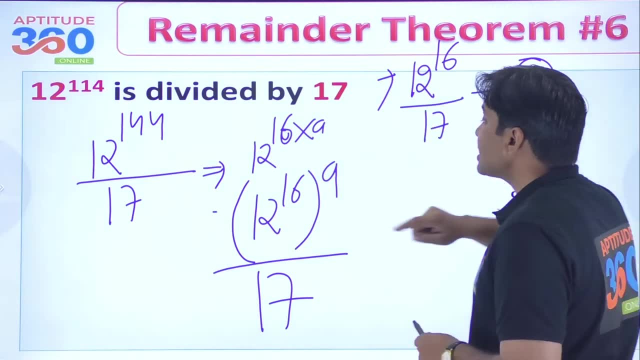 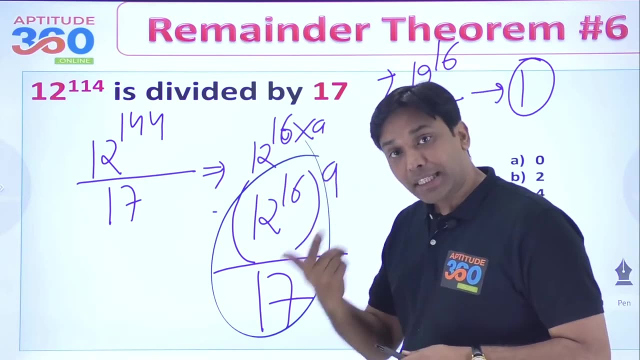 this entire is to power 9. now this number is getting divided by, this number is getting divided by 17 and if this is happening over here, if this is happening over here, this number, this thing, is giving you 1 as a remainder and this entire thing is getting multiplied 9 times. 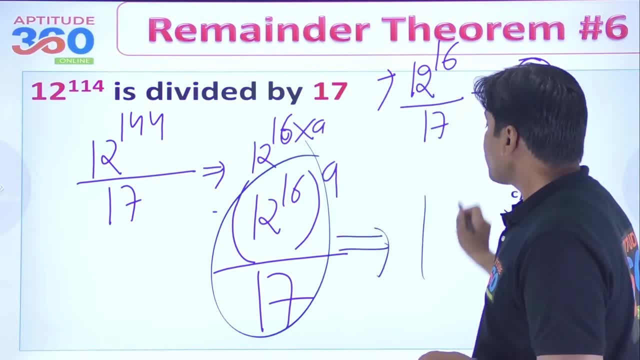 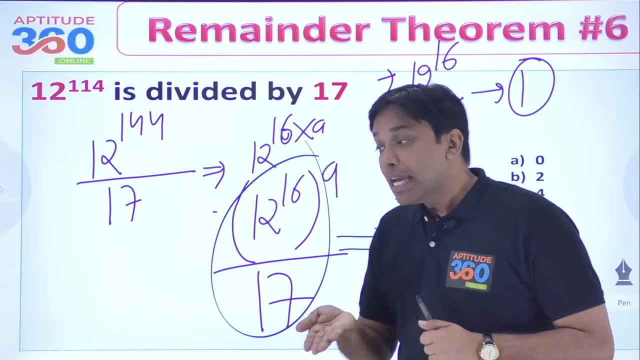 it does not make a difference. so what is the final remainder? the final remainder is coming out as 1. is that ok? so every time, what we are saying in Fermat's Little Theorem, that this which should be in the base, or which you will divide. 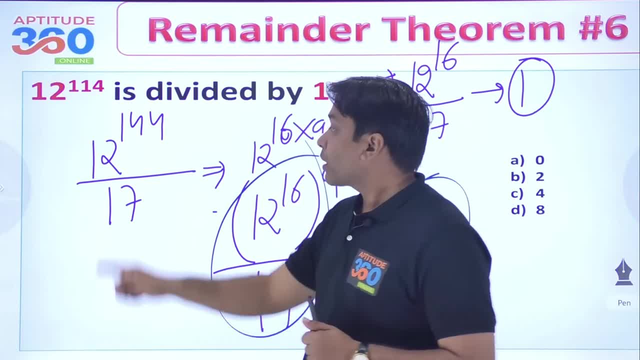 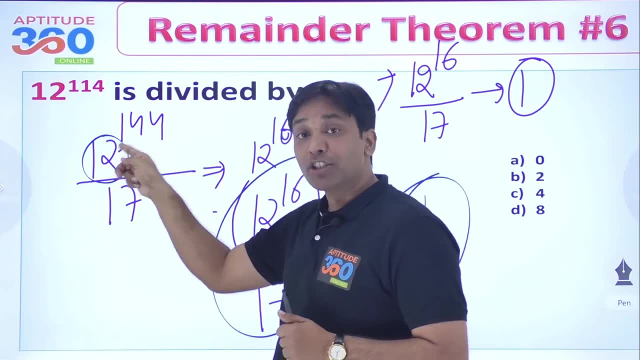 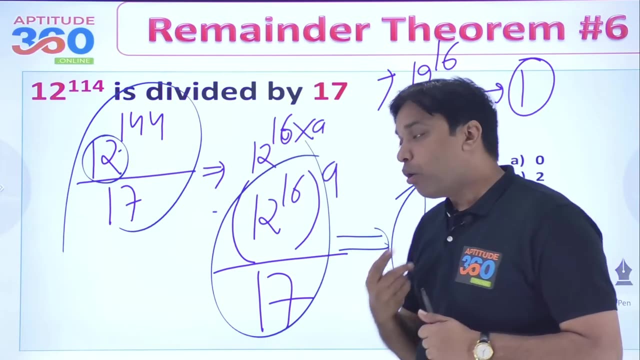 that must be a prime number. this number over here must be co prime to 17 means this number should not be in the table of 17 anywhere. so what you will do is you can simplify this. ok, now solve this one. this one is 6 is to power 59. 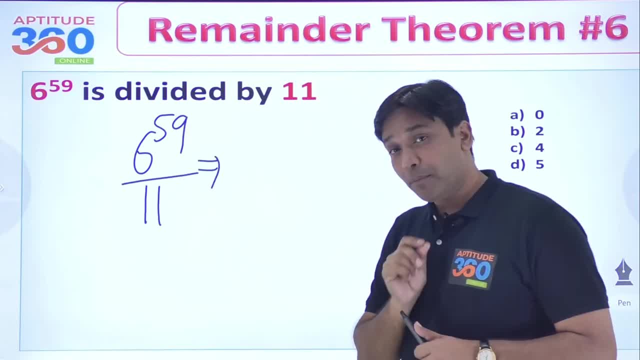 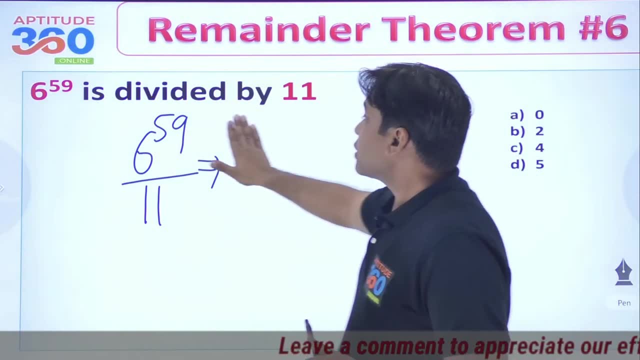 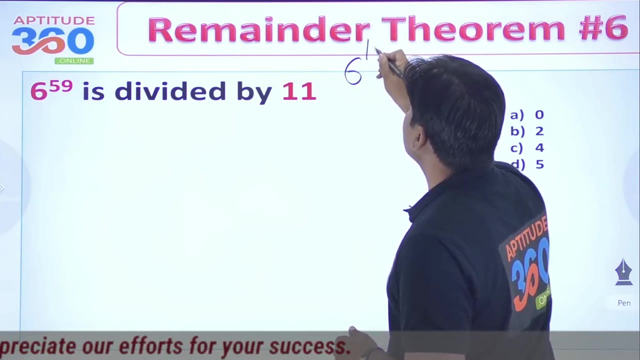 divided by 11. what do you think should be the answer? now, this is kind of a better problem. to solve this problem, what is that we should be doing? we know- for we know this thing for sure- that 6 is to power 10. 6 is to power 10 divided by 11. 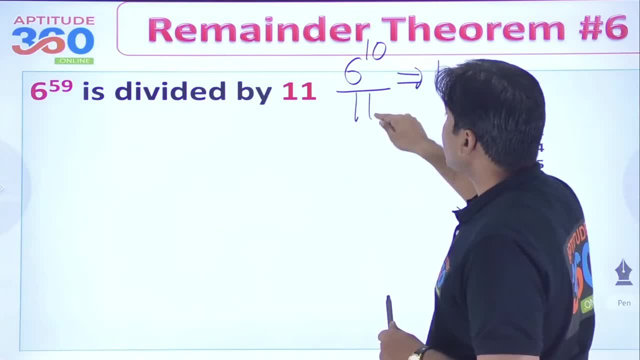 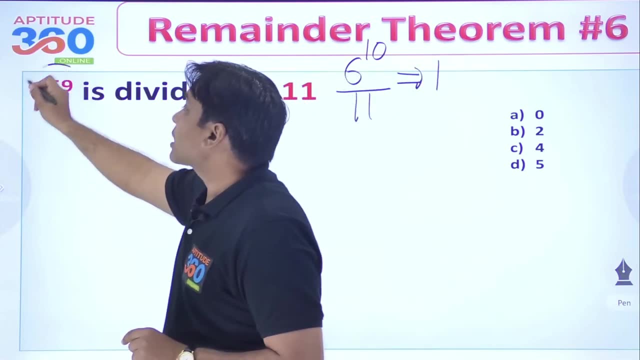 will give me 1 as a remainder. is anybody understanding? 11 is a prime number, 6 is co prime to this and that particular thing will give you 1 as a remainder. but then they are asking you: 6 is to power 59. so can we say that? 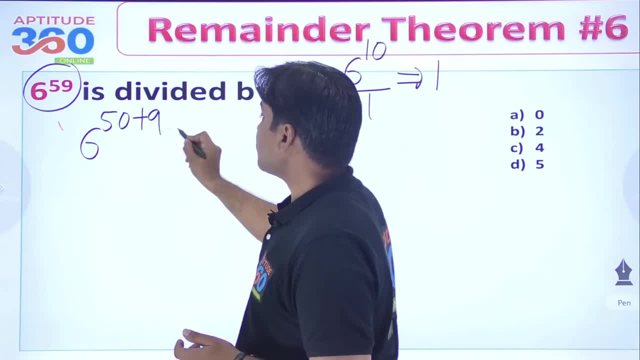 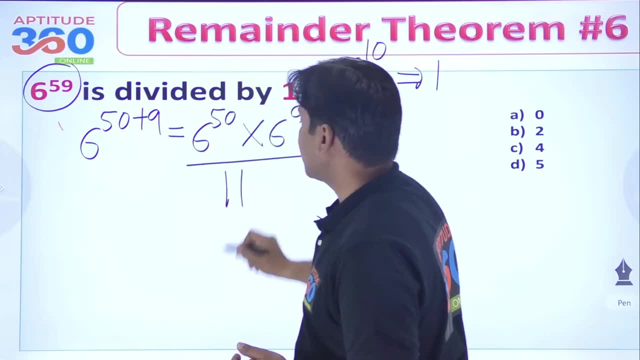 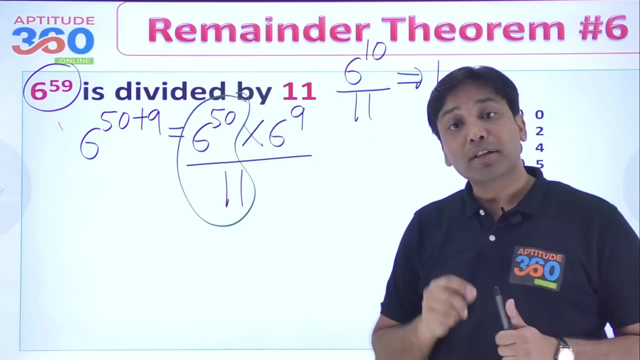 this is going to be: 6 is to power 50 plus 9, so that will be 6 is to power 50 into 6 is to power 9. this divided by 11, right, and if that is happening, this remainder necessarily will be 1, because that is. 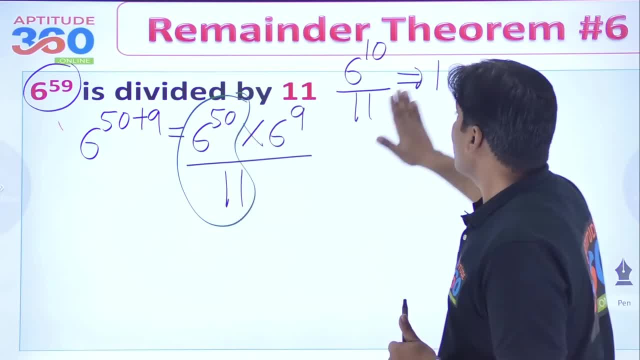 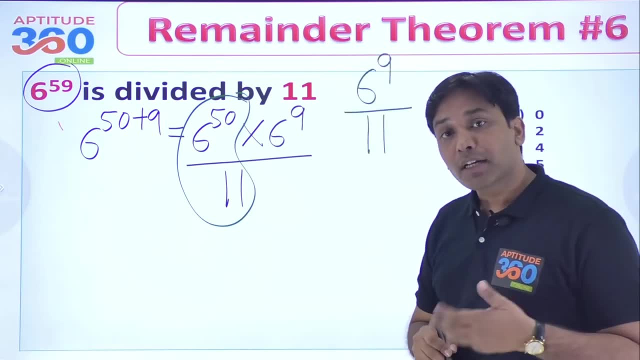 10, 10 into 5, so that remainder is coming out as 1. so what exactly are we left with? we are left with 6 is to power 9, and this number is getting divided by 11. so now what will we do? we will simplify this. 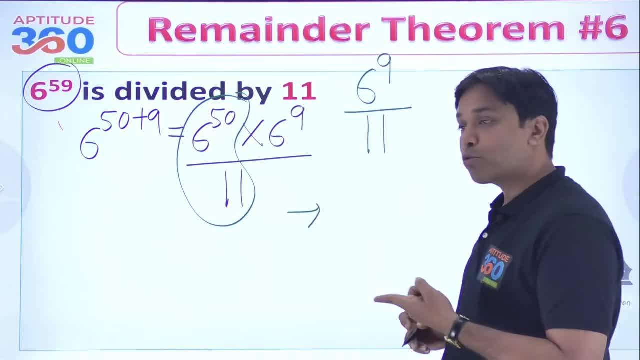 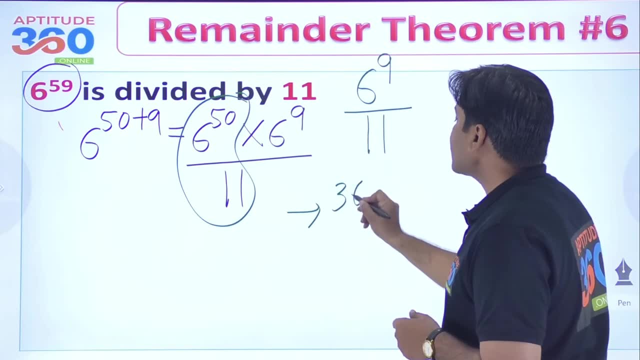 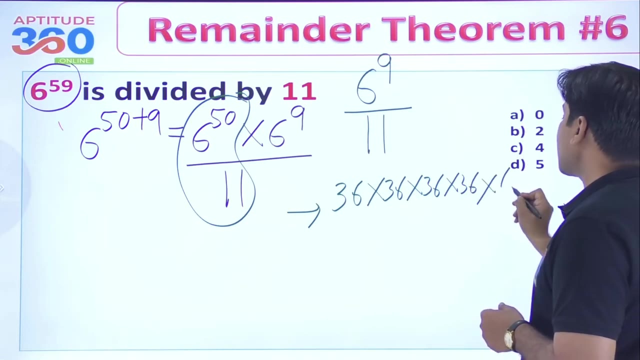 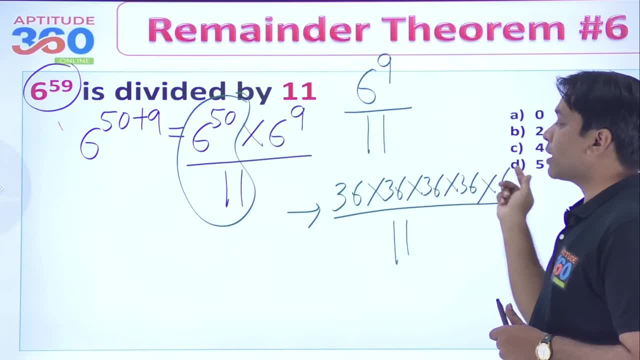 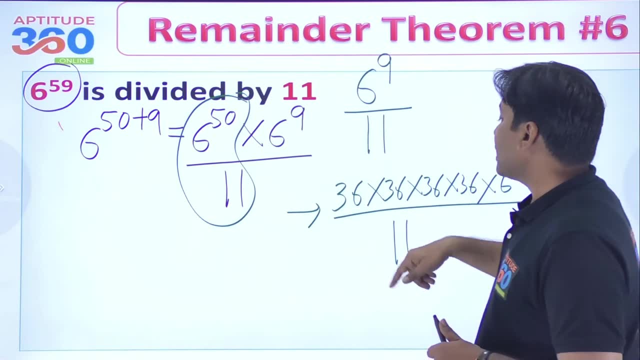 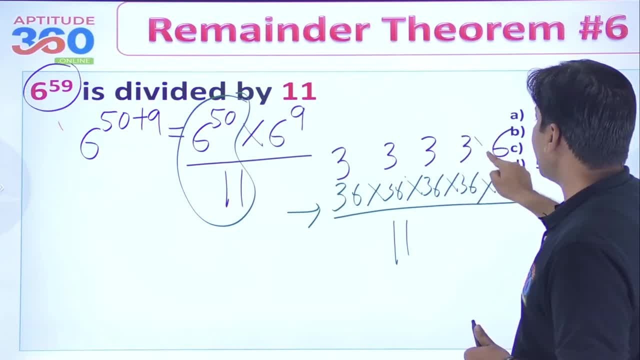 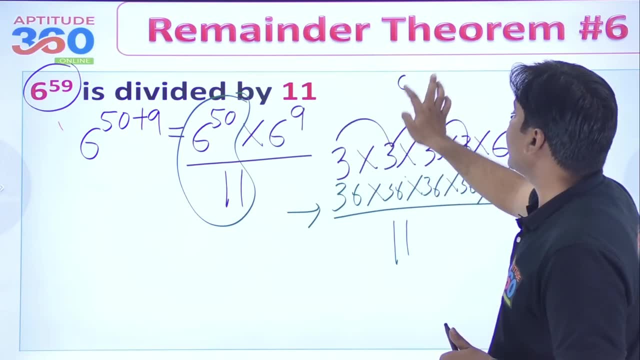 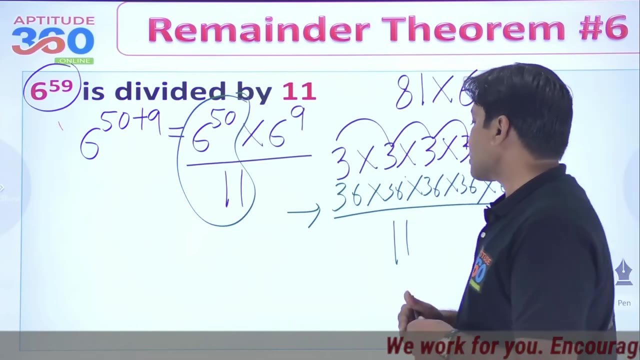 this remainder will be 3 and this will be 6. only then we will multiply this. if you have multiplied these 4, then what will this be? this will be 81 and 81 into 6, something like this: 81 into 6 will be. 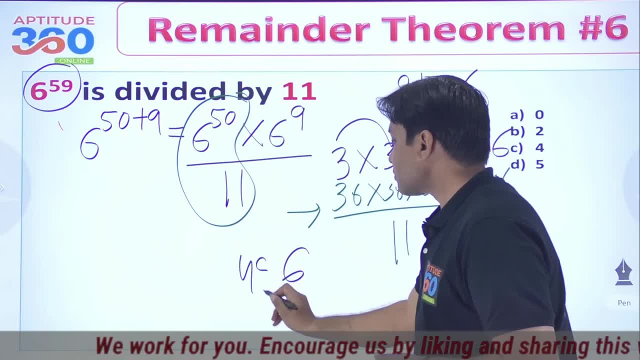 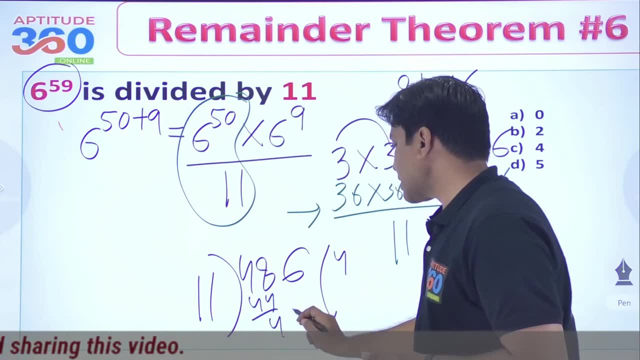 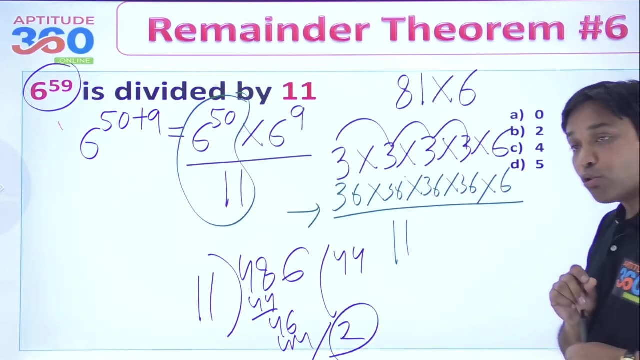 this is 6 and 8. 6 is 48. this is the number, and divide this by 11, so that will be 44 and 46, and it will also be going to 44 times and, and if you simplify this thing, your remainder will be coming out as 2. 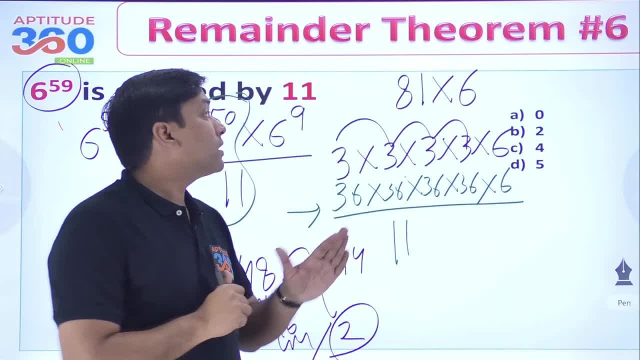 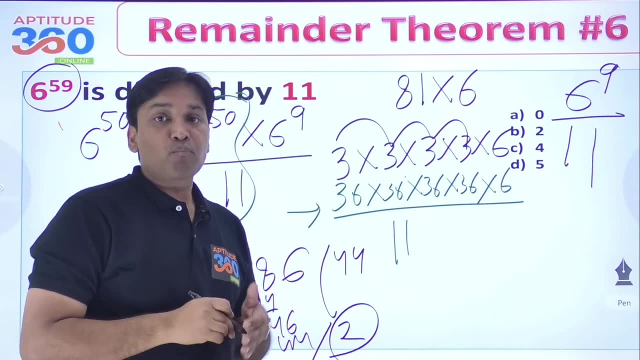 what did you do? 6 is to power 9. we didn't have any idea that 6 is to power 9. 6 is to power 9 divided by 11. how will we simplify this? to simplify this, I told you there is a simple way. 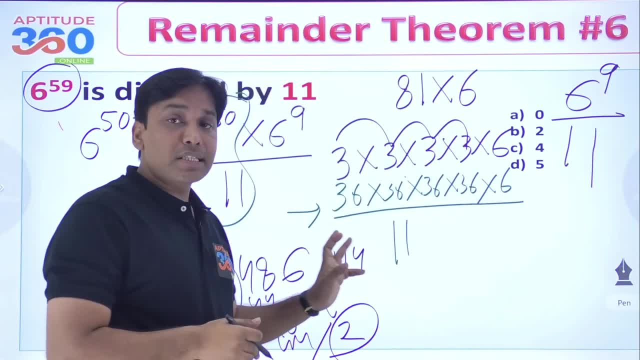 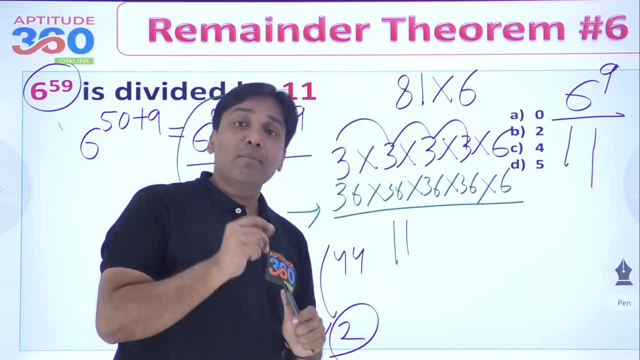 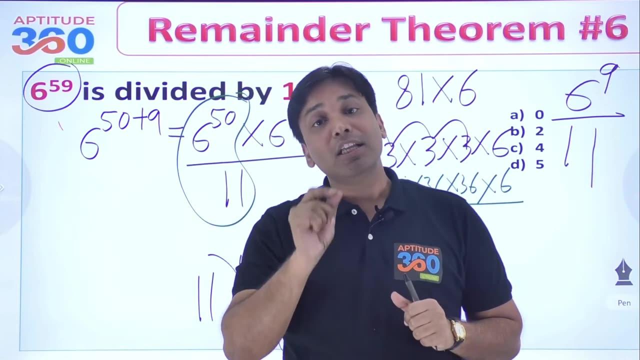 I did it like this. you can use any other way. but having said that, the answer will be coming out as 2. so this is the whole theorem. but every time what we are saying in the Fermat's theorem, the denominator which you will be dividing, the number necessarily will happen. 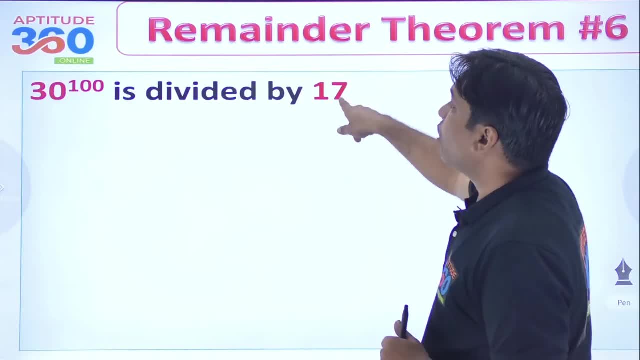 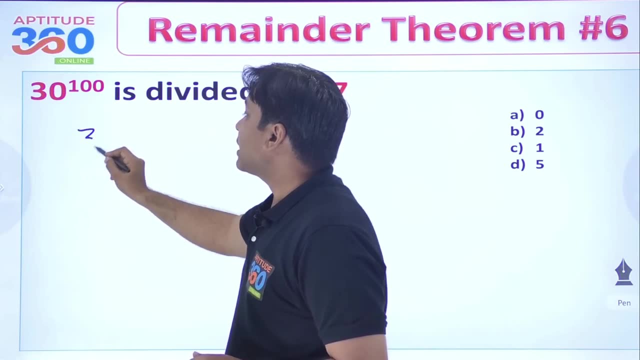 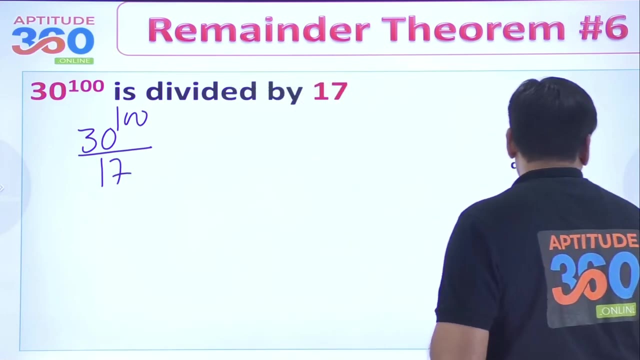 to be a prime number. so how about this one? so 3 is to power 100 is to power 17. if we want to simplify this, we can say that this number is to power 100 is to power 17. now what you do is first write this in a small form: 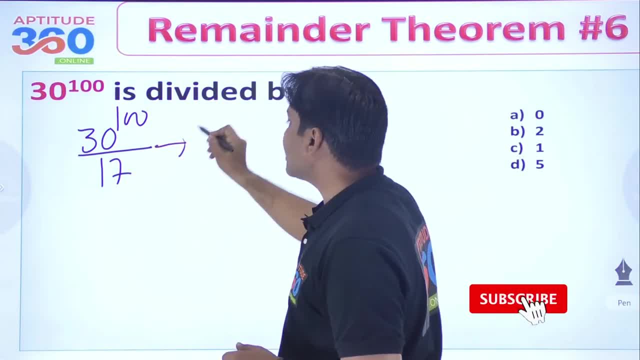 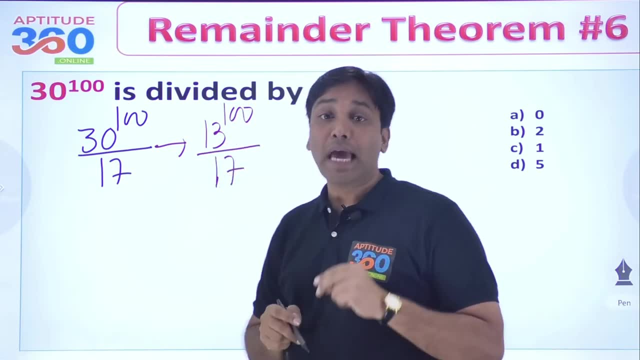 by writing in a small form you can write the numbers correctly. so this will be: 13 is to power 100 upon this number. now everybody must be understanding why am I writing this as 13 is to power 100? now what will happen? what will the Fermat's theorem say? 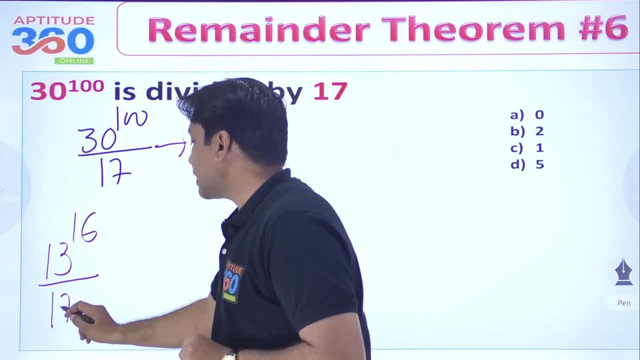 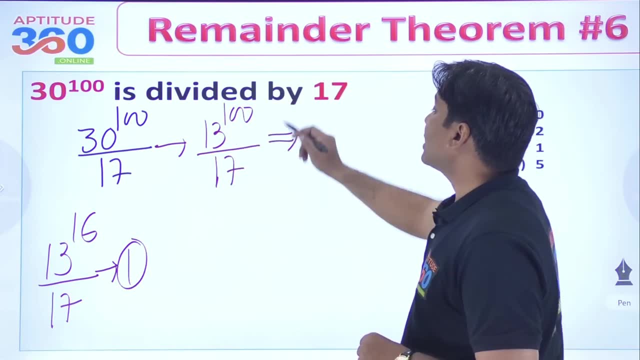 13 is to power 16. divided by 17, this remainder is coming out as 1. is this ok? and over here we have got 100, so I will write 100 as 13 is to power. 96 into 13 is to power 4. 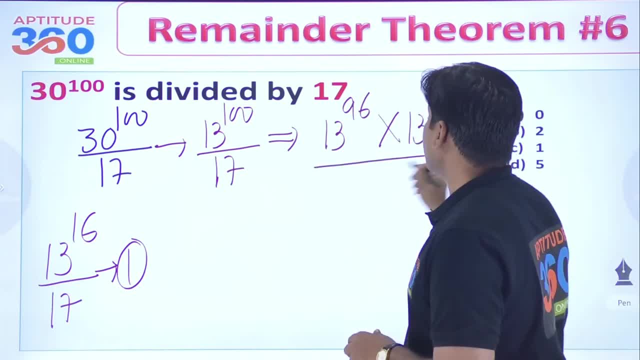 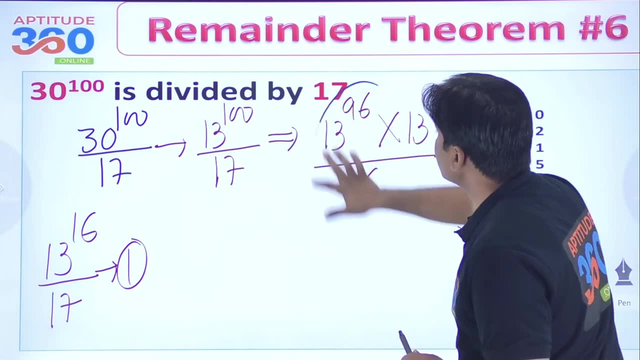 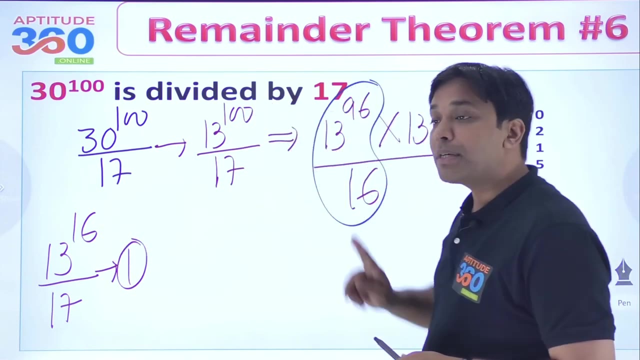 because- and over here this is 16, and now you understand that this has been simplified- this entire remainder will be 1. why it is going to be 1? because 96 is 16 into 6. 96 will be 16 into 6. so what is that we are left with?